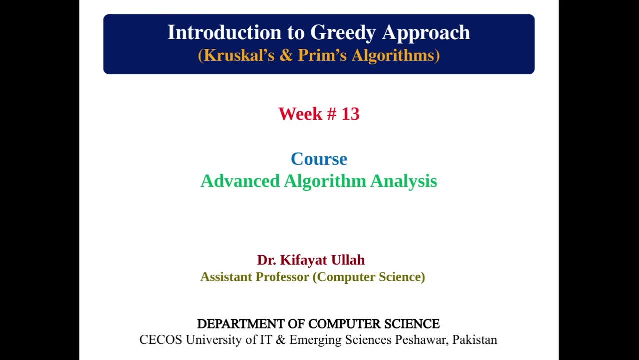 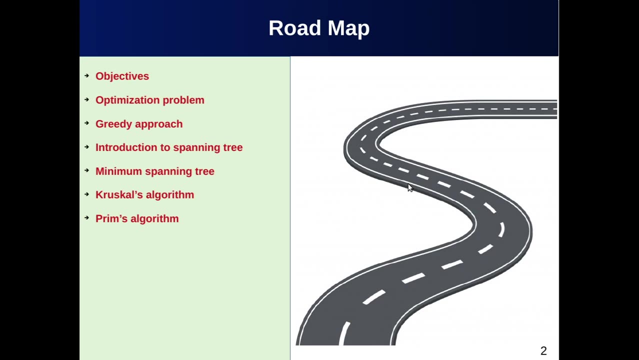 In this lecture we are going to study another very interesting and important topic, which is known as the Greedy Approach, The roadmap for today presentation. as usual, we will start with objectives of the lecture – what you are supposed to learn at the end of this lecture. 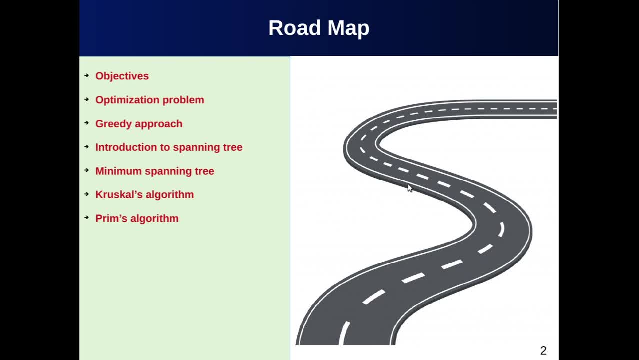 After briefly describing the objectives, we will shift our attention to the optimization problem and then the approach which is used to deal with it, that is, the greedy approach. Then we will describe the concept which is known as Spanning Tree and Minimum Spanning or Cost Tree. 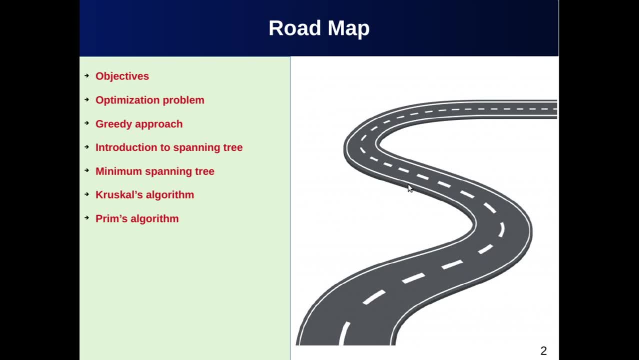 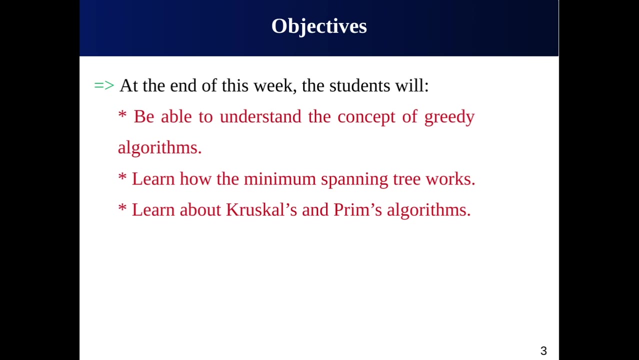 And then two algorithms For finding the Minimum Spanning Tree. there is Kruskal Algorithm and Prim's Algorithm. This is the brief agenda for today's lecture, The objectives, as I just mentioned. at the end of this lecture, you would be able to: 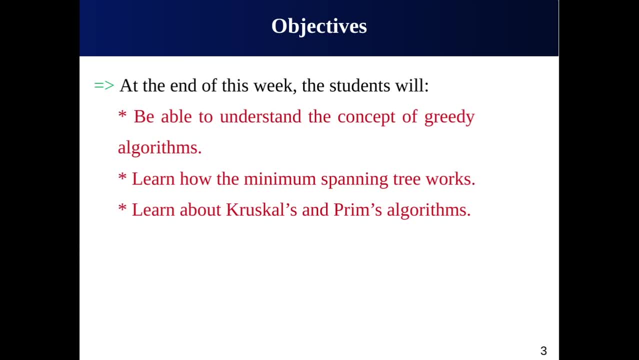 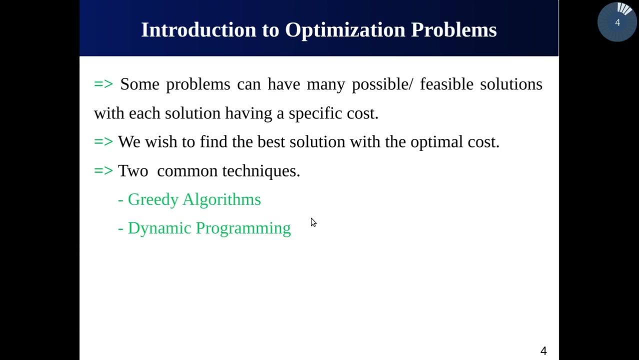 understand the concept of Greedy Approach and also you will learn about Minimum Spanning Tree and two algorithms for finding the Minimum Spanning Tree, that is, the Kruskal and Prim's Algorithm. Before going to start the concept of Minimum Spanning Tree, let me introduce what is an 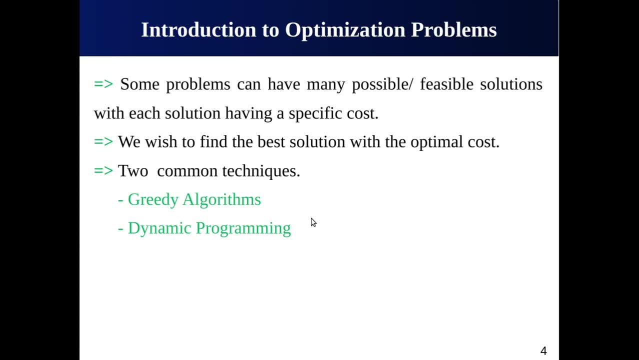 optimized problem. In the field of algorithm analysis, some problems can have many possible, or you can say feasible- solutions, And with each solution having a specific problem. Let me introduce what is an optimized problem In the field of algorithm analysis, some problems can have many possible, or you can say, feasible. 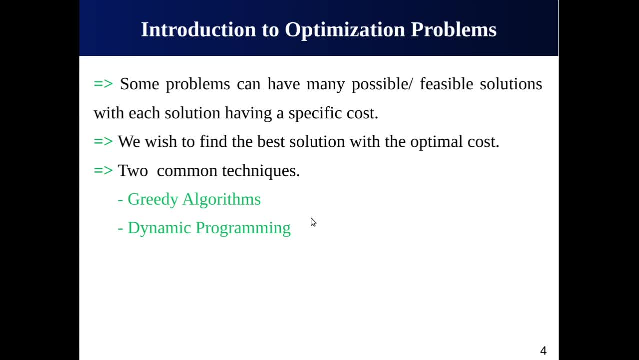 solutions. It is one of the very few opposed to the Frequency vulnerabilности check mushrooms of the system. we already have choppers and the number of scripted, You can say that a set of choices must be made in order to might, in order to solve the problem. 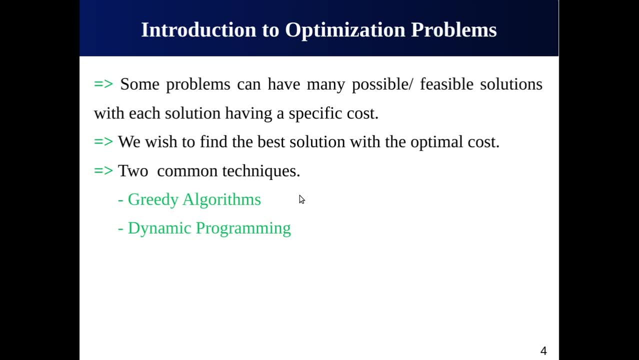 in order to arrive at an optimal solution. The optimal solution? in some cases it could be the minimum possible value, or in other cases it could be the maximum possible value of a problem subject to some constraints. For optimization problem, we actually have two common techniques available. The first technique is known as greedy and the second is known as the dynamic programming. 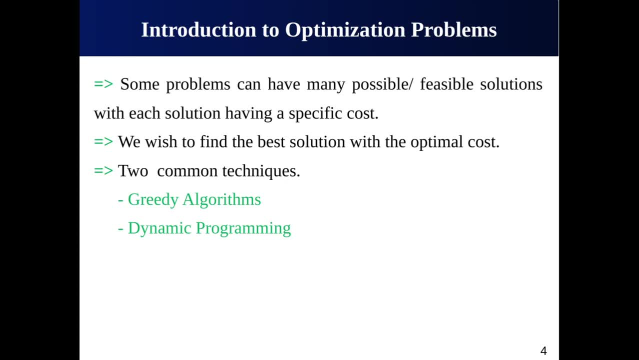 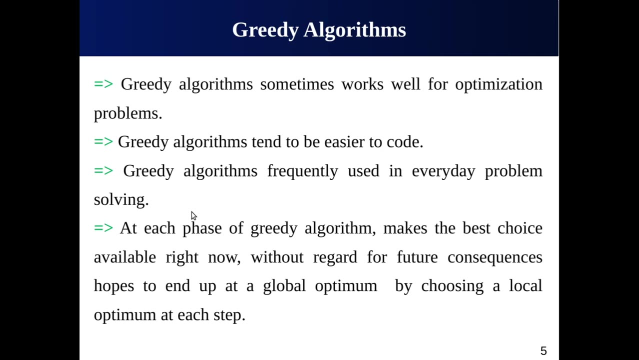 The focus of this lecture is greedy algorithm, but we will also shed some light on the dynamic programming concept. Let us start with the greedy approach or greedy algorithms. Actually, greedy algorithms, sometimes they work very well For optimization problems and they are- comparatively they are- easier to understand. 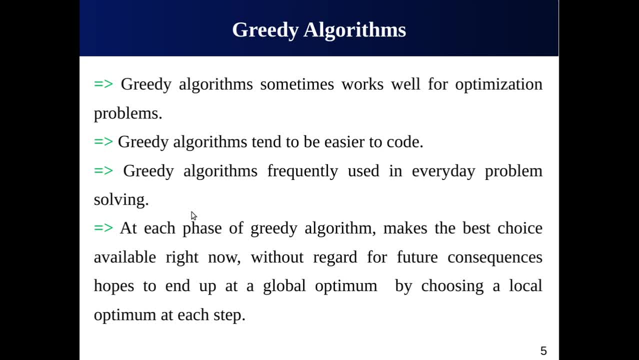 and easier to code or implement as well, and it is. this approach is frequently used in our everyday problem solvings. Let's suppose you are choosing a job and then you are going to to make your final decision. That decision could be based on the greedy approach. 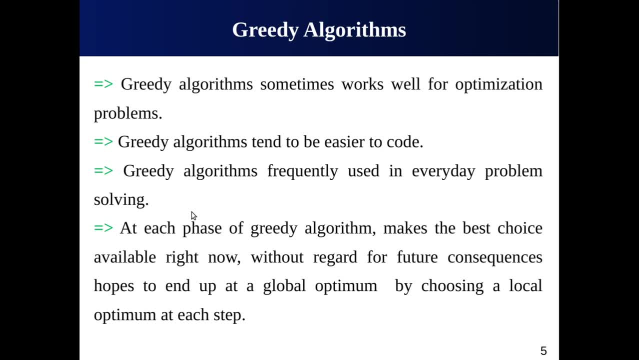 Or you are traveling to another city or another destination and you are going to find the most suitable route for yourself depending on several factors or, as I just mentioned, constraint, like the traffic condition, conditions on the road, the weather, the condition of the road itself, 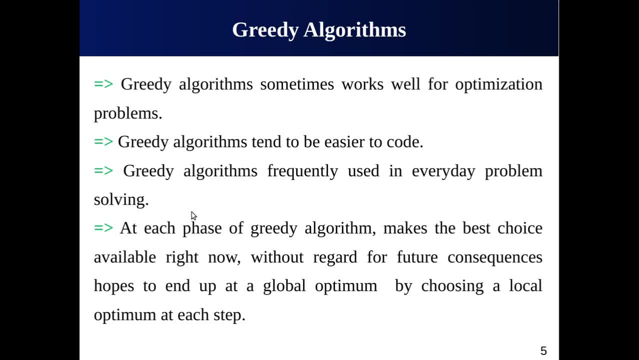 the time required to reach to the destination, and factors like it influence our decision. In a similar way, if you are playing the cards, game playing cards- and then you want to place a card, Certainly you have different options, choices, available Now how you will make your decision it. 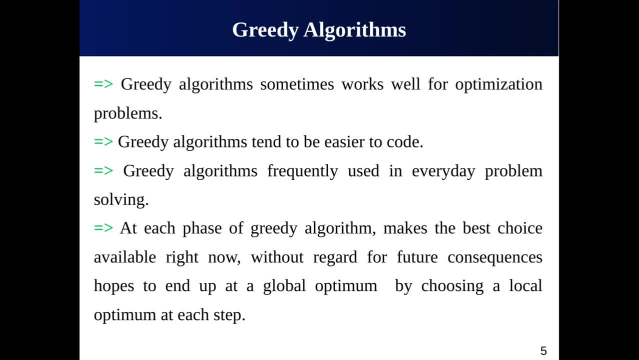 could be based on the greedy approach. Or if you are investing in the stock where you will invest your money to earn more profit, It could be based on the greedy approach. So a greedy algorithm actually works in different phases And at each phase of the greedy algorithm we makes the best choice available. but at the moment, right now, 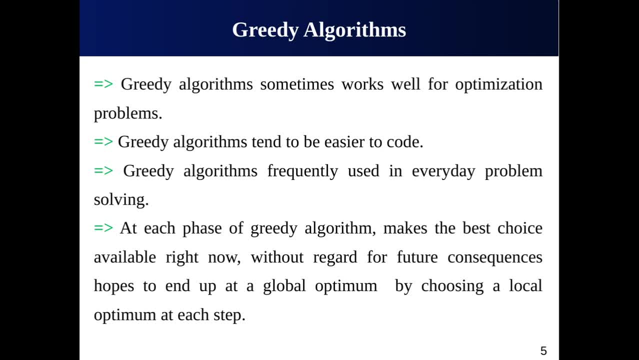 That is the property of the greedy algorithm: We always, always want to make the best choice in the current situation, current circumstances, without regard for future consequences, And then we hope to end up at a global optimum solution by choosing a local optimum solution at each step. So, in summary, in the greedy approach, we always try our best to make the best choice. 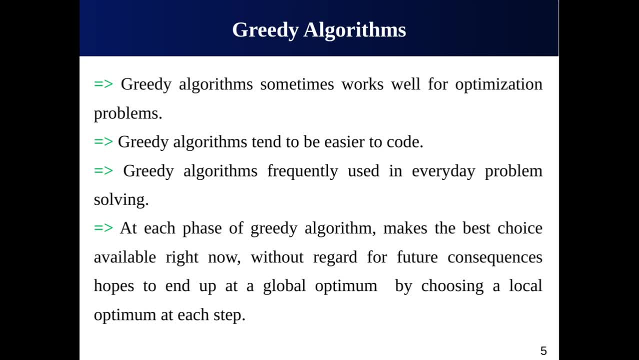 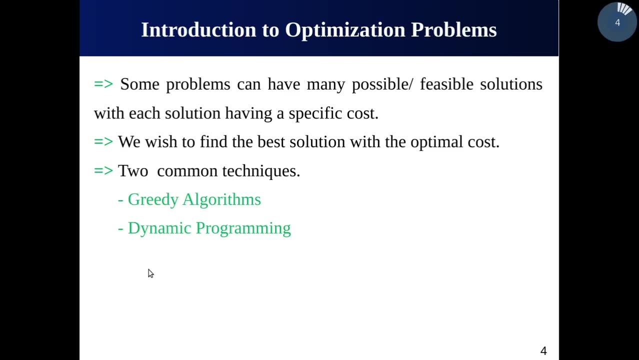 available right now, in the current circumstances, without regard for the future consequences. We will come back to the greedy approach in a moment And we will study in more details about this, But first let us see what is actually the dynamic programming approach. As I just mentioned, we have two different techniques available for optimization. 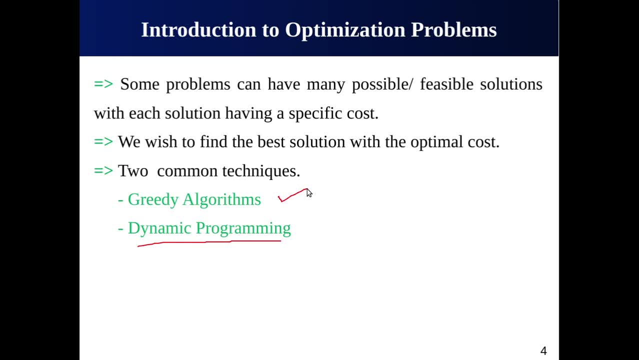 problem. The first one is greedy algorithm, which is going to be the focus of this presentation, And the second approach is known as dynamic programming. Dynamic programming concept was introduced in 1950s by Richard Billman. It is actually mostly. in most cases this technique is applied to optimization problem like the greedy. 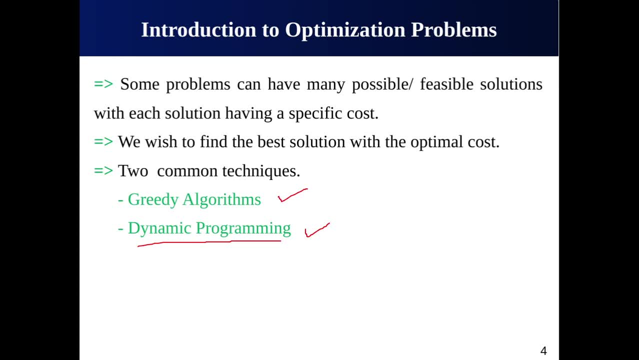 approach problem. Okay, let me tell you one thing: that the dynamic programming. actually it doesn't refer to computer programming, But it is a strategy for designing algorithms And, to be more technical, it is actually a meta technique, Not an algorithm that we use. 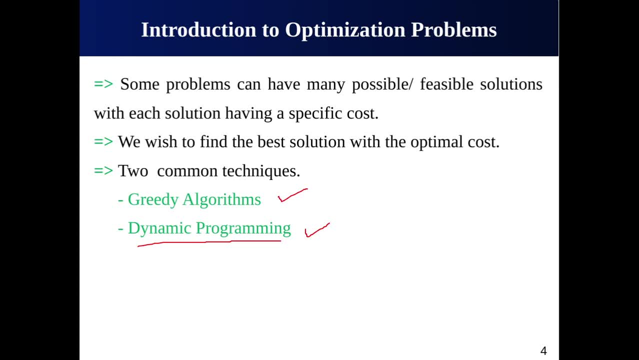 That we follow to find the optimum solution to a problem. Okay, dynamic programming actually solves every sub problem just once. We make a choice at every step towards the solution, And our choice depend on solutions to their problems, And in dynamic programming, the approach that we actually use is a bottom-up solution approach, Or 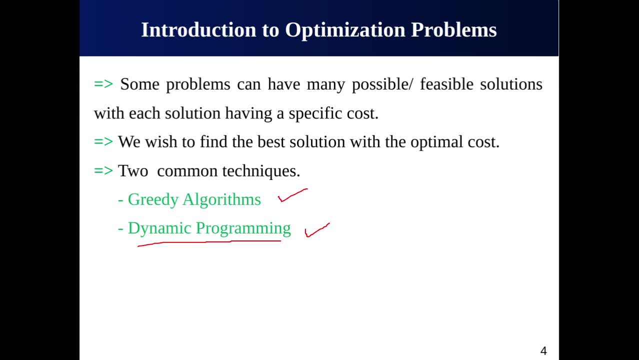 say from, we are moving from smaller to larger sub problems. you might be thinking or comparing the dynamic approach with date of the divide and conquer approach, because in the divide and conquer approach, as we saw in case of merge, sort, quick sort, binary search, it also solves problems by combining solution the problems in order to elaborate further the divide and. 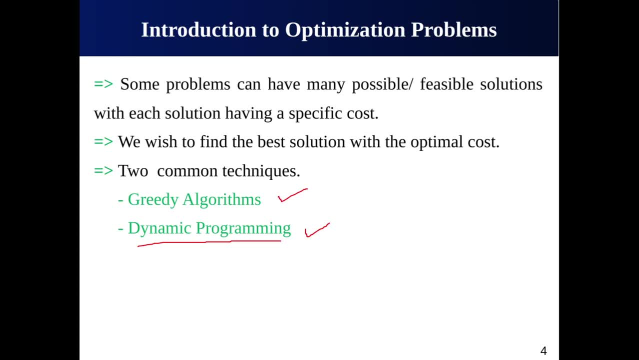 conquer approach. we partition the problem into independent the problems and then we solve the sub problem recursively and finally we combine their solution to solve the original problem. same is the case with dynamic programming. however, dynamic programming is applicable when the sub problems are not independent. sub solutions are the solution to the sub problems. 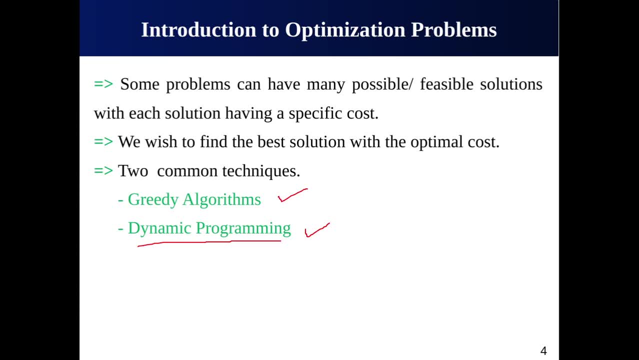 or the sub problem itself. they are dependent on one another. you decide from this difference. we also have another difference between the divide and conquer approach and the dynamic programming approach, and that is that the divide and conquer approach is actually a top-down approach, while on the other side, the dynamic programming is a bottom-up approach. let 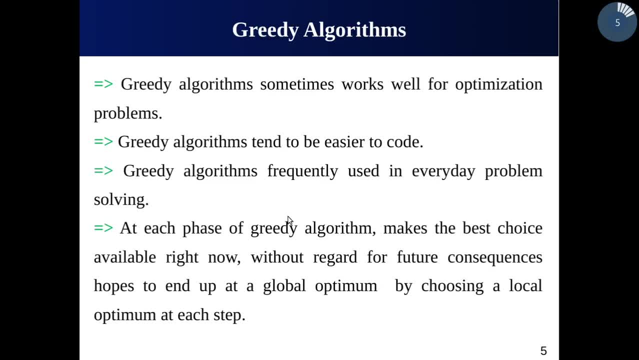 us bake our attention to the greedy algorithms. I'm supposed that you are familiar with the word greedy. if not, let me elaborate it by using a reference to a study that what. it was conducted by the researchers in the University of Oxford and the study was published in natural communication. and the study brings out: 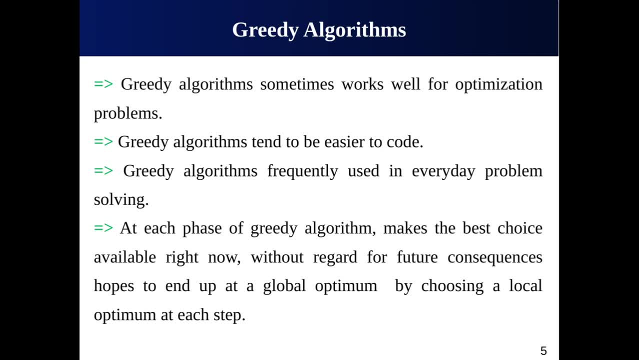 an interesting fact and the fact was very simple and it proves that greedy is something which is good and the higher radicals structure structured communities. that class at the top of of the community. in the community it actually takes care of the lowest in the hierarchy and they also compete. 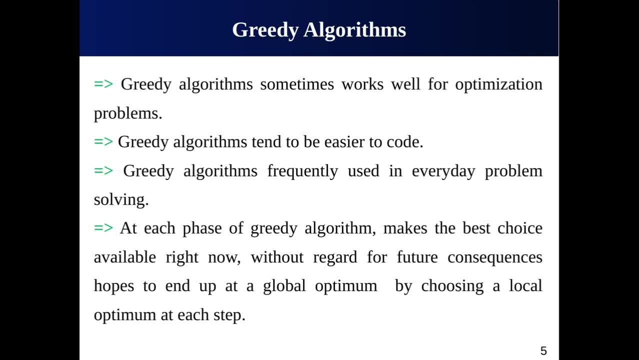 with the classes at the top of other groups. actually, we see some gradin S here, and greedy S is good and bra الذ Cuz. actually we see some gradins here and gradient math is good- good for those that are superior in their groups and also for those that are at the lowest. 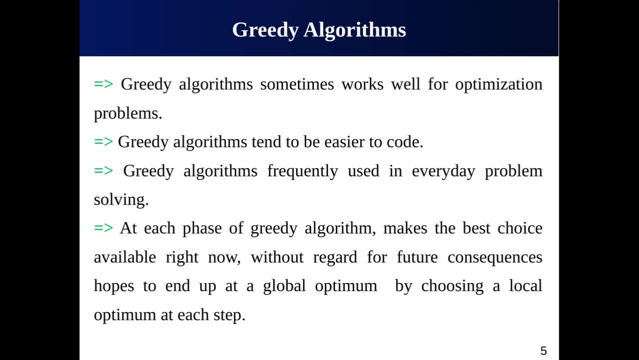 level in that group. you can also find several examples of this approach in our society, even in our religion. it has been said that you can compete with your fellows while learning something that is allowed. that type of greediness is allowed. even our economies run on the basis of. 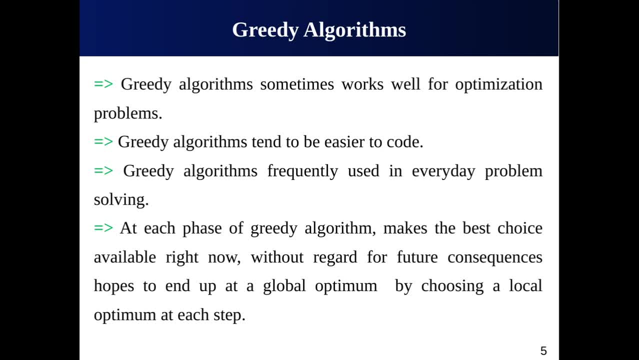 this greedy approach and also the companies. they are able to survive because of this greedy approach. everybody wants to select the best approach towards the solution. even those who rule us follow this greedy approach. so it's up to some extent that greediness is good and it the rule. also apply on algorithms. 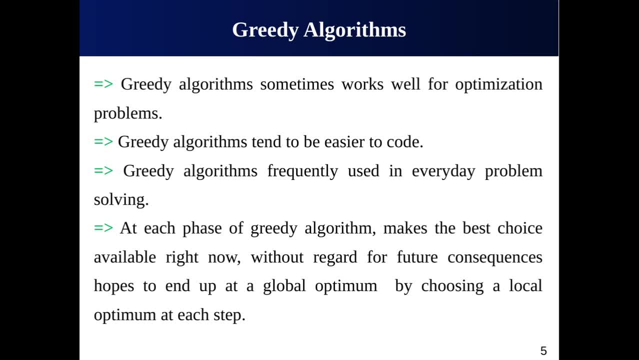 you solving problem-solving approach, date incorporate, you can say- a pinch of greedy readiness. it actually helps us to attain the goals in a better way and perhaps in less amount of time. so this greedy approach of solving a problem calls for the selection of most promising intermediate solution at date particular time. 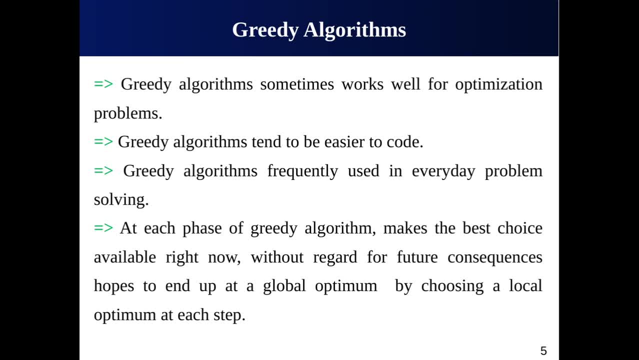 you, or at date instance of time. the intermediate solution which seems promising at a point might not, may might not be good in long terms. remember, in the greedy approach we always try to select the best solution at date, time or eight date, particular instance of time. but maybe in long terms, our solution is not good in order to solve a problem. uh, with greedy approach, 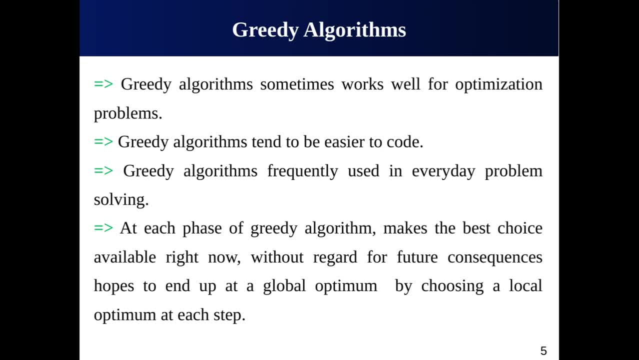 we actually select an input and if the solution satisfy the the greedy goal that we have set for it, then it is taken in the solution set. otherwise it is left. so we have some goals in our mind and then we select a problem and to solve that problem by this greedy approach, we select an input. 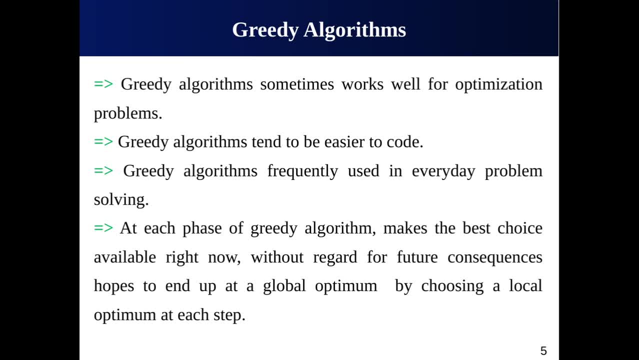 if the solution satisfy our goals, the greedy goals, then it is taken in the solution set. otherwise it is left. okay, so in conclusion, the greedy algorithms work most of the time. however, they are not always optimal because we always consider the solution that are best at date particular instance of time. let us move our attention to this. 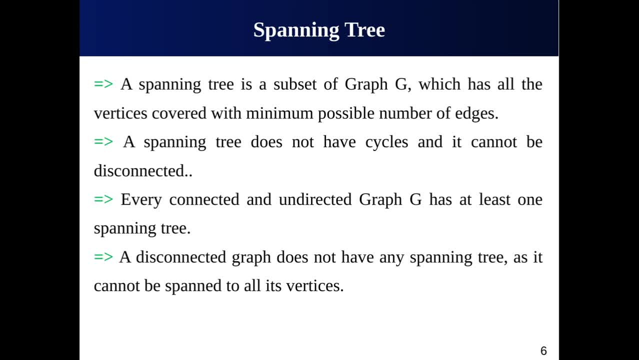 funny, a spanning tree concept. a spanning tree is a subset of a graph. for example, the graph is denoted by g. so spanning tree is actually a subset of a graph. however, it must satisfy some properties. what are those? the spanning tree in a spanning tree, all the vertices. 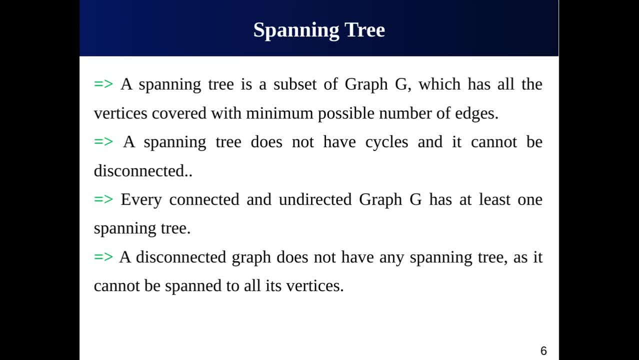 are covered with minimum possible number of edges. that is the basic property of a spanning tree means. the first point is that it is actually a subset of a graph. second thing: all the vertices of this subset of graph. they must be covered mean they must be connected with minimum possible number of edges. 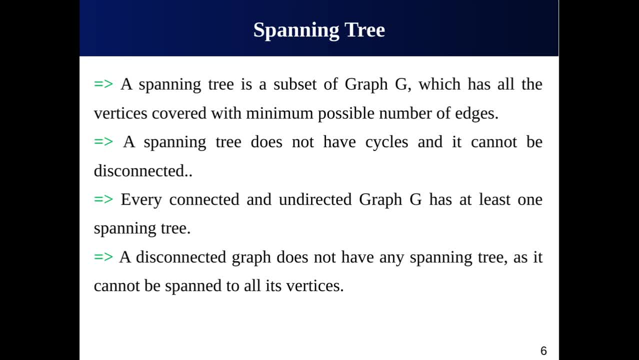 if we are interested in finding the optimal solution. in this case, the optimal solution is to reach to the destination with minimum possible number of edges, or you can say the cost, minimum cost. another thing which is important for a spanning tree is that a spanning tree does not. 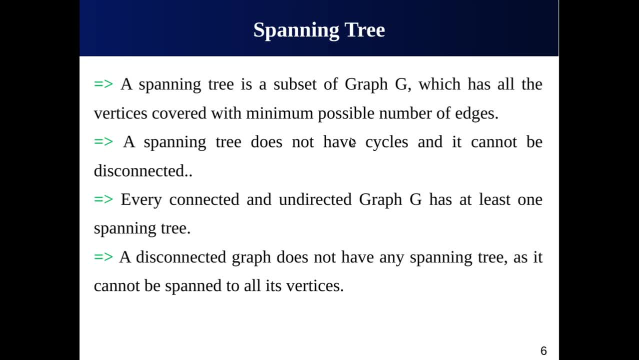 have any cycle. this is something very important. cycling- the concept of cycle we have already studied in the graph. terminologies having an ending point is same, which mean it is a loop or a cycle. in case of expanding, tree spanning tree will not contain any cycle, and another thing is that it can not be disconnected like a forest. 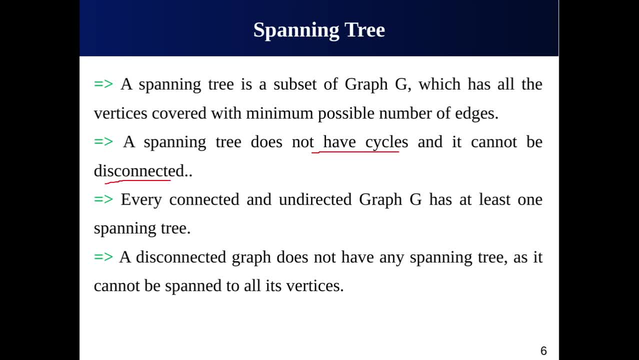 where one or more than one nodes are not connected to the rest of them, of the nodes are, or to rest of the graph subgraph. so all the vertices must be connected, must be reachable, and by this definition and by from these, from these properties, we can draw a conclusion, and the conclusion is: 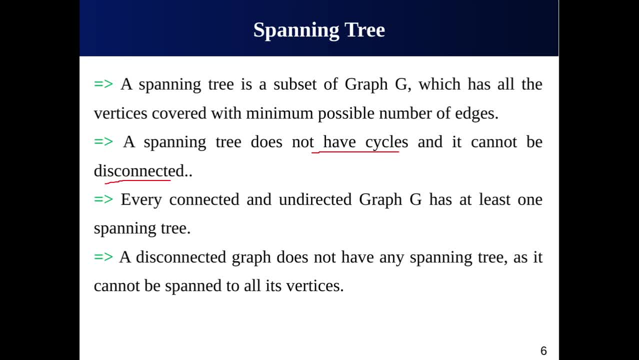 they to. every connected and undirected graph has at least one spanning tree plus they are connected with one another and there is a path from source to destination. so the conclusion is that every connected only connected, not. the definition will not be applicable on the unconnected or not connected graph, and also the graph should be undirected. 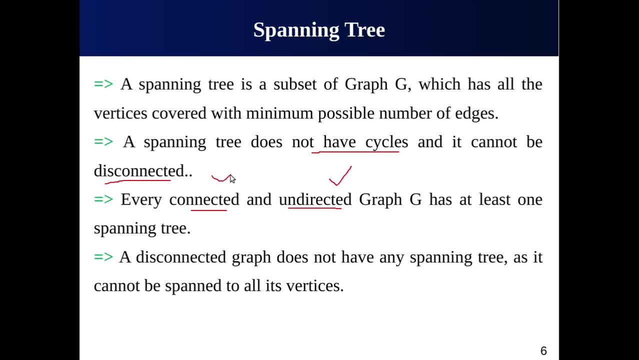 so if a graph is undirected and it is fully connected, then you can say that there exists at least one spanning tree and also the graph should be undirected. so if a graph is undirected, spanning tree at least mean it could be 1, 2, it could be 3 and so on. 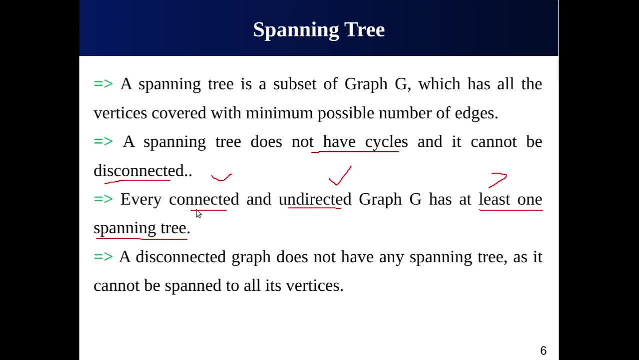 okay, I talked about connected graph. now what about disconnected? a disconnected graph does not have any spanning tree because it cannot be spanned to all 8 vertices. remember, it must be connected. so if a graph is disconnected then it cannot contain any spanning tree. let us see some general properties of a. 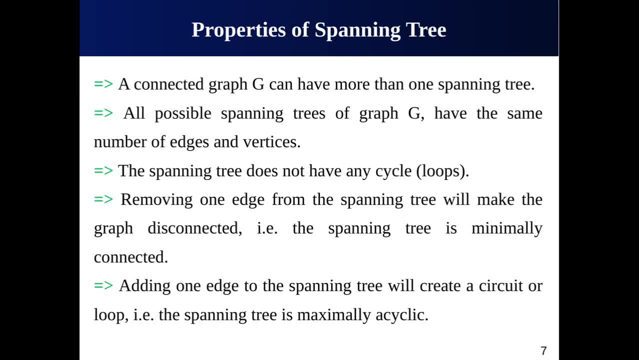 spanning tree. we now understand it, a graph, which is a connected and undirected, can have more than one spanning tree. it lead to some properties and these properties are for connected graph, undirected. the first property is that a connected graph can have more than one spanning tree, and we just saw it. it is possible. 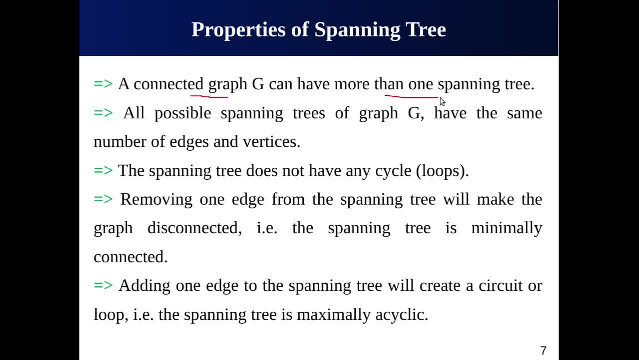 for a connected graph to have at least one spanning tree. that is the first property. similarly, all the connected, all the possible spanning trees of a graph, they must have the same number of edges and vertices. for example, you have created five spanning trees from a graph. now all these spanning trees must have. 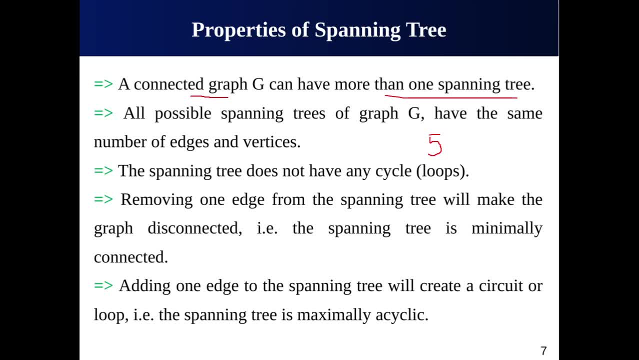 the same number of edges and vertices. edges mean the links that actually connect the vertices, and vertices also mean the nodes or extension nodes that connect the vertices working same way. similarly, for example, if we insert a spanned tree, we can create an extra spans working in which we create a密 thread. so by contributing, by adding a more, 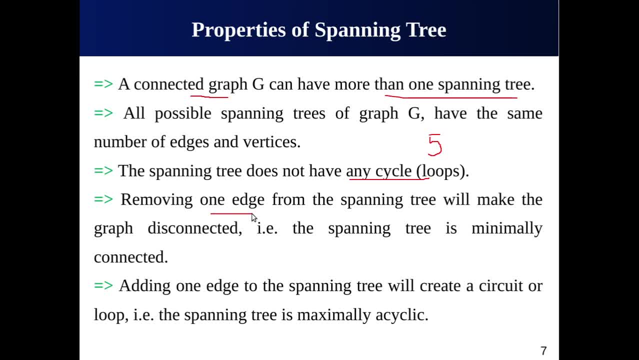 specific wor. nevertheless, this essential, we are generated a final loop of shared percentage or expressions which can be exactly Fer Länder, so I will just take some. but if you remove any one edge from the tree, then the graph will become disconnected. what does it mean? it means that the spanning tree is now minimally connected, so this is another property. 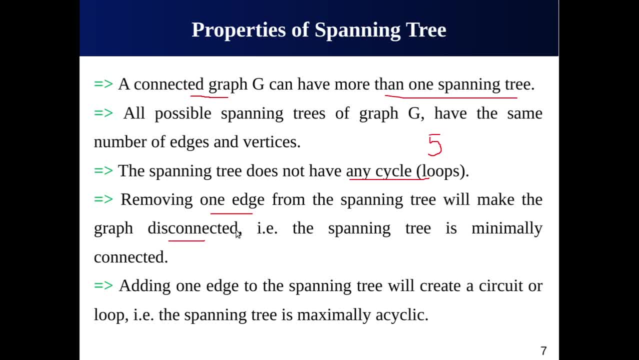 that the spanning tree is formed in such a way that removal of any one edge from the tree will cause the graph to be disconnected. and finally, if you add one extra edge to the spanning tree, what will happen? actually, it will create a loop, or you can say a circuit or a cycle. and now the 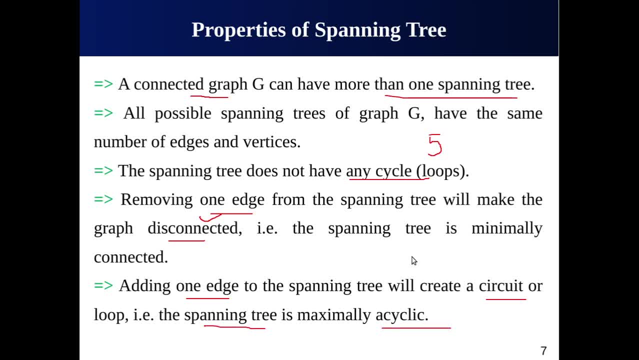 spanning tree will be acyclic. the opposite of cyclic is acyclic. so removal will violate the property of the spanning tree as well as addition. addition of a new edge will also violate the property of the spanning tree. in summary, the spanning tree of a graph is actually a connected- uh, a connected- graph. 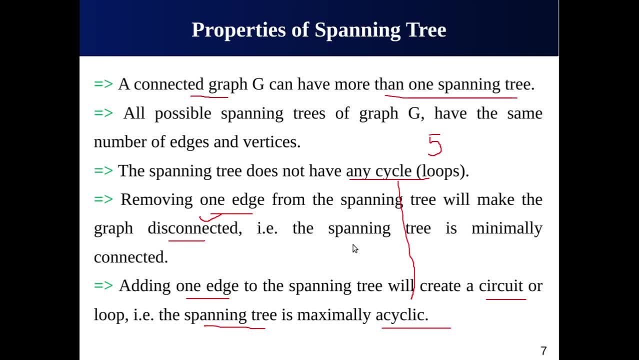 undirected graph with no cycles and no loops, so it is actually a graph g which you can represent, like vertices and edges, the spanning tree. here is a graph of a graph which is actually a graph of a graph, a connected subgraph, with no cycles and all the vertices of the tree are covered, are connected. 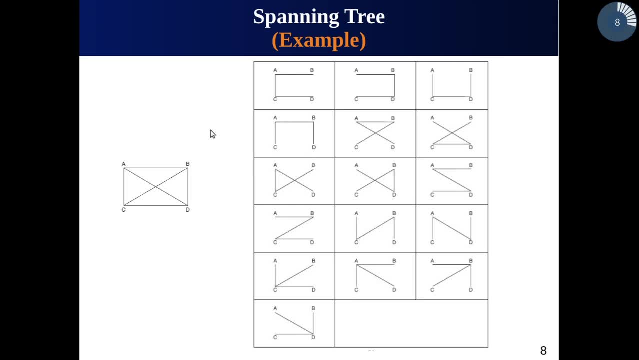 let us see an example clarify the concept. we have a graph, which is mentioned here, and we are trying to identify all the possible spanning trees of this graph. we have four vertices here. the vertices are a, b, e and d and they are connected by using a different links and we are going to form the spanning tree for this. 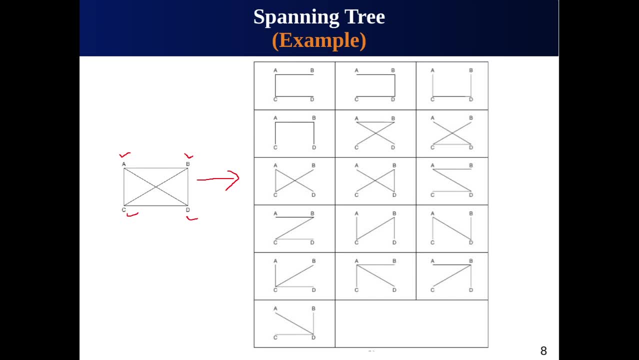 graph. yes, we just saw that more than one spanning tree are possible. so how many spanning tree trees actually do we have here? total of 16.. all these are valid spanning trees. you can see that the number of vertices and number of edges, they are actually the same. 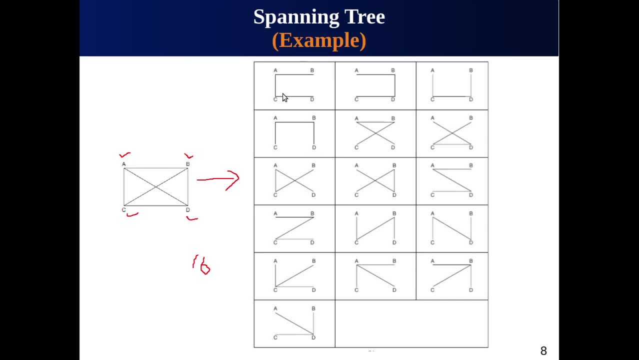 number of vertices are four everywhere. every single spanning tree has four vertices and the edges connecting these nodes is also the same. three here, three and three. that is the property of the spanning tree. now there is only one half of this story, one side of the picture. the whole exercise is to select and optimum. 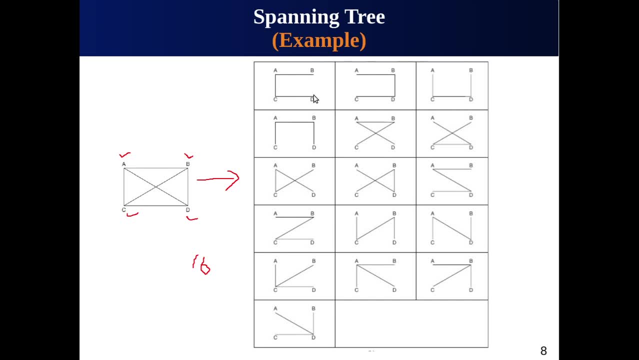 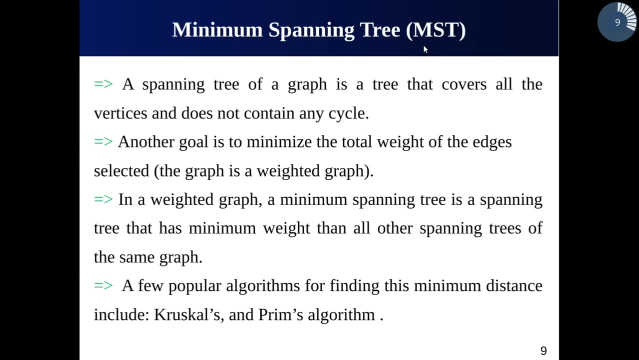 solution. from all these possible solution, we would be interested only in one single solution, and that solution must be optimal, must be the best solution available in all these possible. for that we have to use another concept that is known as MSP, or you can say minimum spanning. let us see what is a minimum spanning tree. 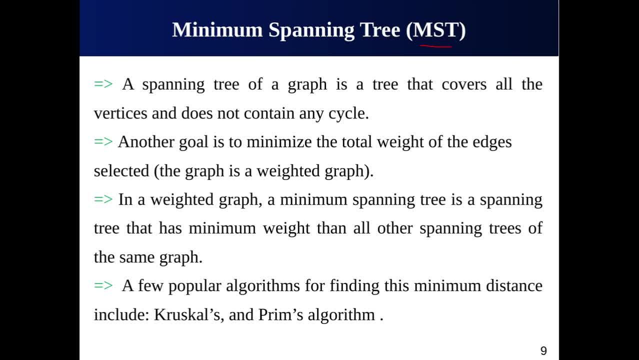 a spanning tree, as we just saw, is a tree. it covers all the vertices and it does not contain any cycle. in other words, you can say that the graph doesn't have any nodes which loop back to itself. starting and ending points, or source and destination are the same. there is not possible. 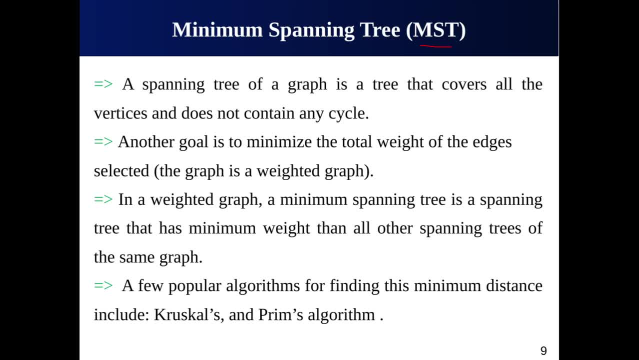 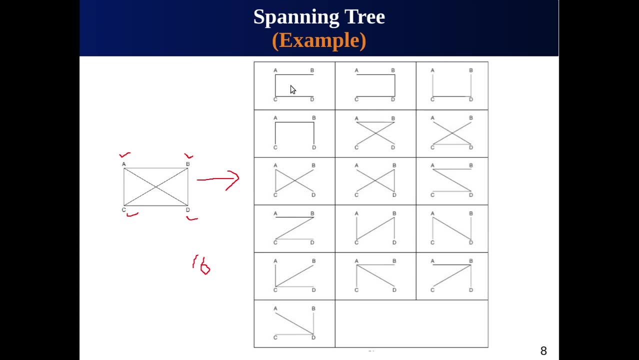 now what if we have a weighted graph? a minimum spanning tree is actually a spanning tree. it has minimum weight. then all other spanning trees of the same graph. let us take another. the same example once more. we have different. you have formed different spanning trees. now the minimum spanning tree among these solution will be the 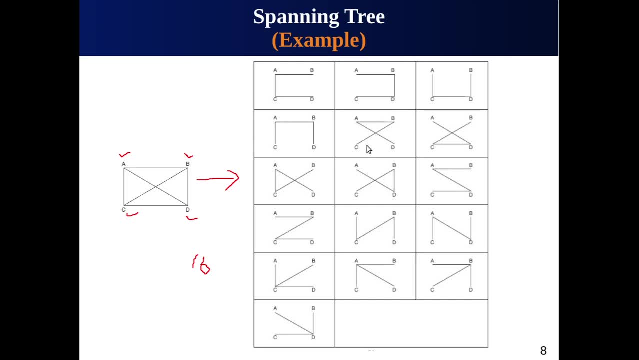 one where the minimum weight is possible, like the tree will have minimum possible weight. for example, the overall weight of this spanning tree is 10. weight would be anything, if you remember the weighted graph. it could be cost, it could be congestion, it could be distance, etc. here we have eight where we here we have six and the total weight here is four. 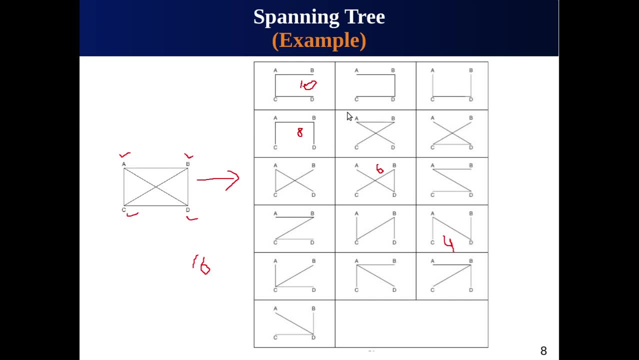 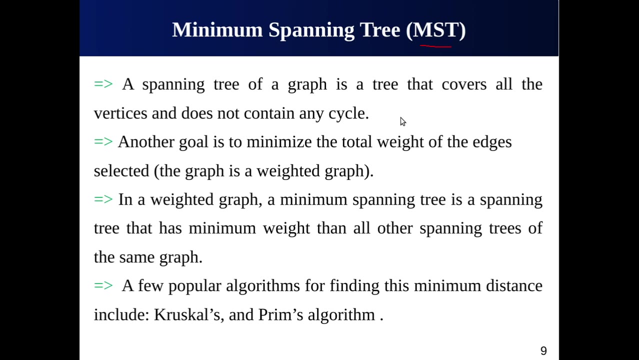 now you can see what is going to be the the best solution in all these cases: the minimum cost, and the minimum cost is four. here we will select this spanning tree and there is the responsibility of the minimum spanning tree algorithm. you can say that a minimum spanning tree is actually a special kind of tree and 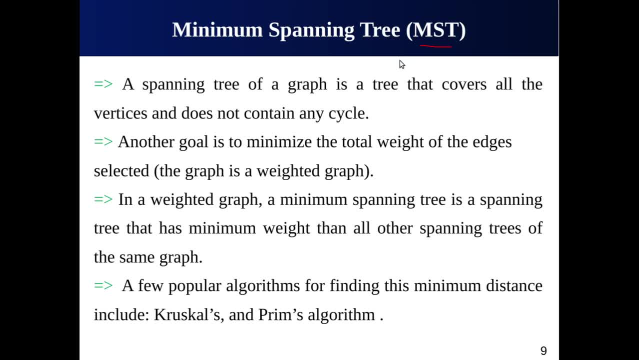 with some properties and the properties are like the tree actually minimizes the length, or you can say the weights of the edges of the tree. in real world scenarios, in real-world situations, this weight can be measured as a distance in the sessions, traffic load, any arbitrary value. 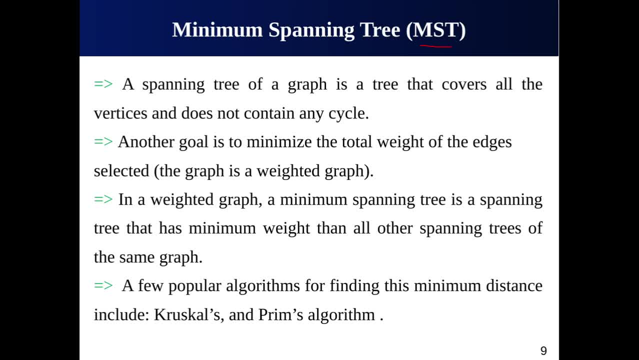 denoted to the edge. take an example. for example, we have a cable company and they want to lay a line to multiple neighborhoods, but they wish to minimize the amount of cable played, and the company will also want to do it because they will save more money by doing so. okay, so they have to. 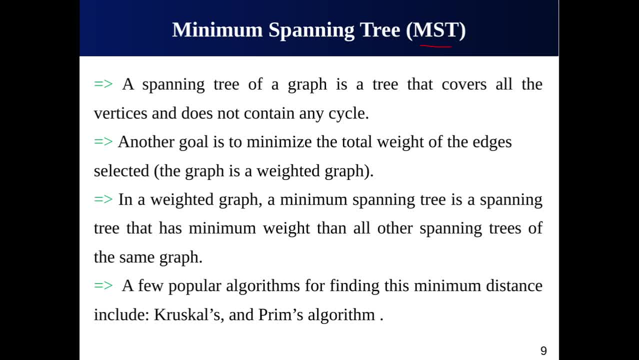 go for a scheme which will actually lead to the deployment of less amount of cable in order to save more money. and there is the same with the minimum spanning tree concept. we are actually interested in finding a solution that will lead to the minimum cost possible, or minimum weight. 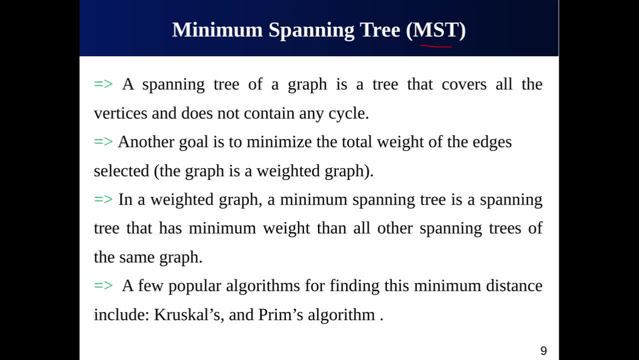 possible in order to source, to save our resources and, for date, a several popular algorithms are available. you can see the different algorithms are available which actually find the minimum distance, and these algorithm include a crystal algorithm and prim algorithm, and there is going to be the topic of 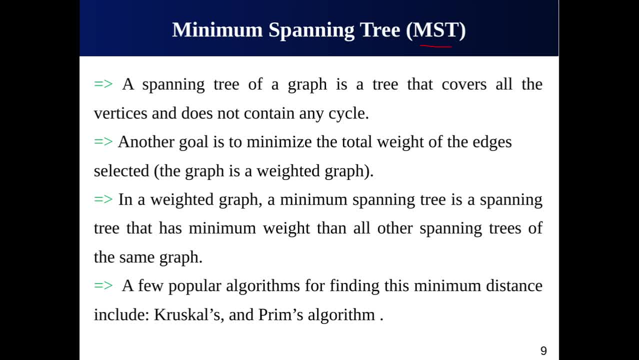 discussion and we will see it in a couple of, in a couple of minutes. what is crystal crystal algorithm and what is prim algorithm? and both these algorithms are used for finding the minimum, to the uh, to the concept of spanning tree, and let me rewind the tree that covers all the vertices. 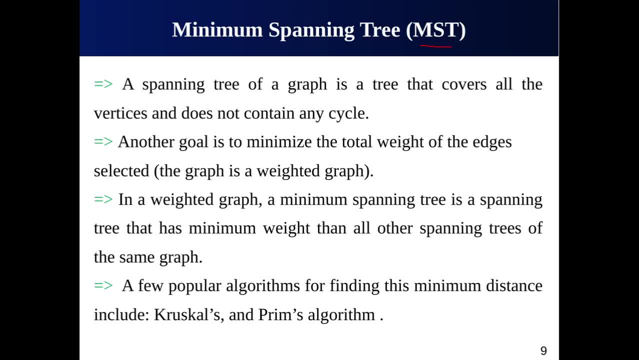 okay, and with no Loop or with no circuit or with no cycle. but besides from this, in most of the practical application, there is another goal and which need, which needs to be achieved, and the goal is to minimize the total weight of the edges selected if it is a weighted graph. but we can use a greedy algorithms, or you can say: 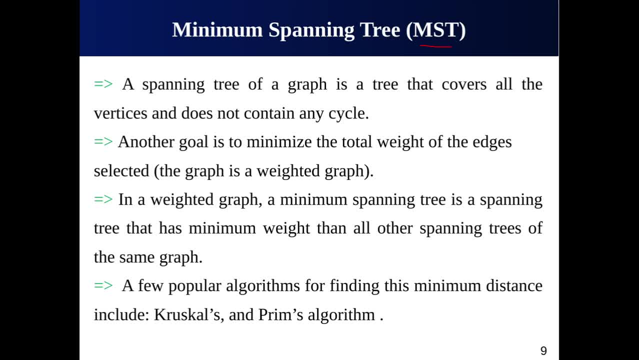 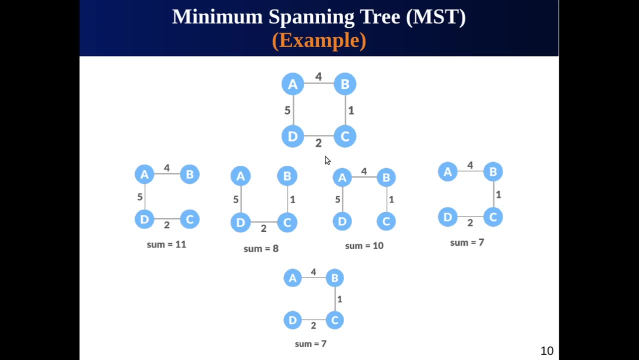 a minimum spanning tree to accomplish this goal, this task. let us see some example to clarify the concept of a minimum spanning tree. the concept can be understood with the help of this example, which is mentioned here. we have an initial graph here. the graph has four vertices: a, b, e and d, and every uh. we have 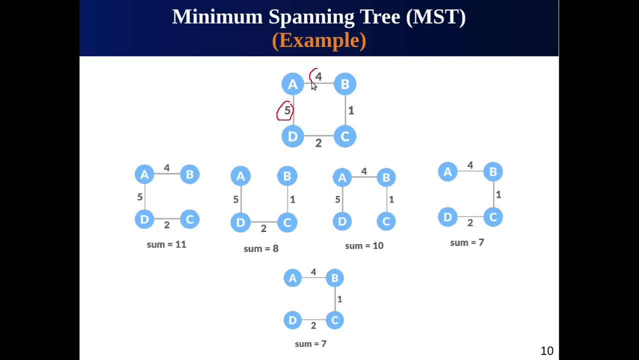 associated a number with each edge, or you can say each link. this is actually the weight about which i was talking. it could be anything. it could be distance between the nodes, can be anything. it could be junctions of on a route, could be two different cities. it could be two computers they want to communicate. it could be. 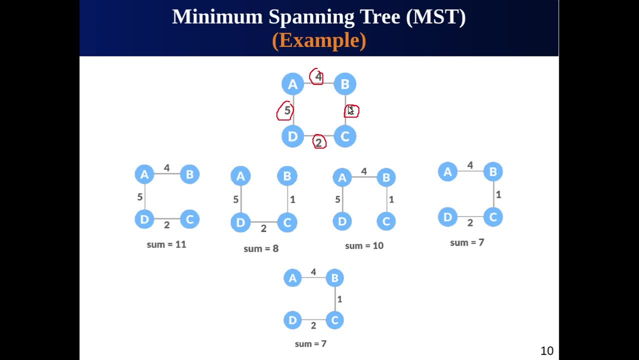 two sensor nodes, anything. and there is the weight, it could be anything again, could be distance, it could be the time required to travel to send a packet. it could could be anything. any arbitrary number. okay now the possible spanning trees for this graph, not the minimum spanning tree. 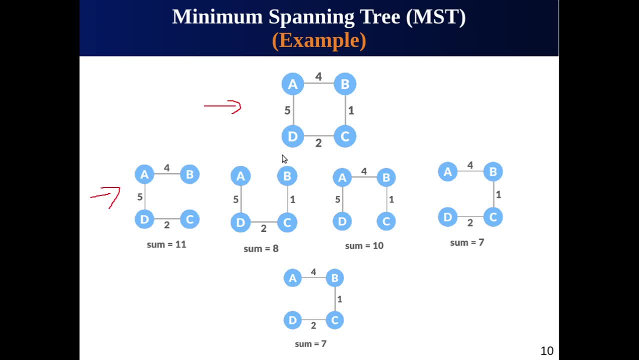 all these possible spanning trees for this graph. they are mentioned here, so we have four spanning trees. now what is the total weight, the total cost of each spanning tree? you have to add the number associated with each link. so here the sum is 11. there is 4 plus 5 plus 2.. here the overall weight, or sum, is 8.5. 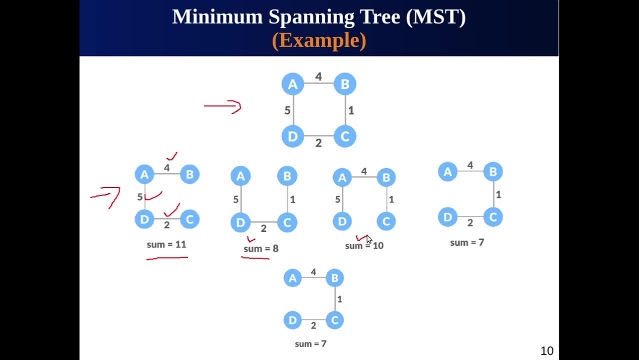 5 plus 2 plus 1, here we have 8, 10 and then finally we have a sum 7.. okay, very simple. the minimum spanning tree from the above spanning tree is the one with the minimum overall weight or cost, and that is 7.. so this is our minimum spanning tree algorithm. 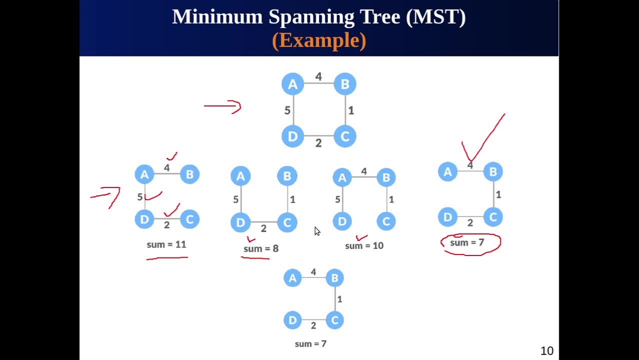 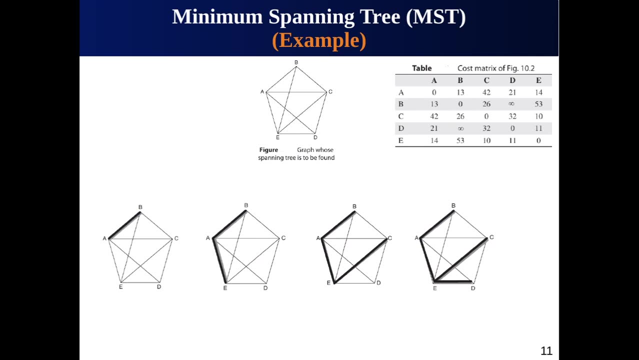 not algorithm, but solution. minimum spanning tree. actually, if this example is clear, that's good. if not, let us consider a second example, a minimum spanning tree, sometime. it is also known as minimum cost spanning tree because we are interested in the cost or in the weight, so you can say a minimum cost spanning tree. 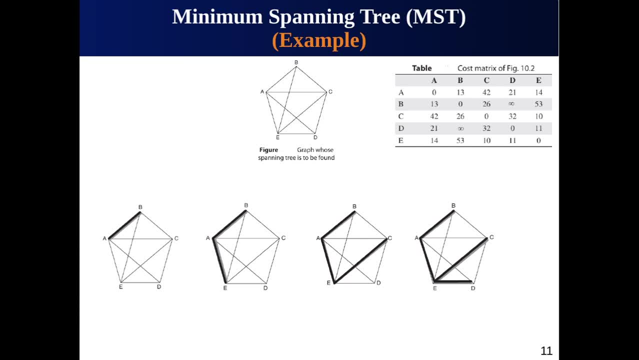 is actually formed from the given spanning trees. let us consider another example. here we have different nodes, five nodes: a, b, c, d and e- you can consider them different cities, and then we have different links connecting these cities. and also we have another component parameter and there is the distance. 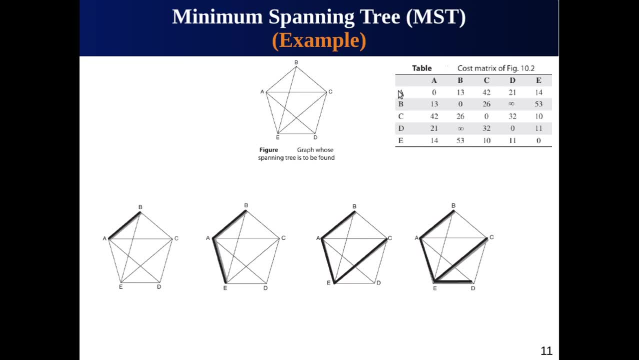 between these cities. for example, if you want to travel from a to a, the distance is zero. but if you want to travel from a to b or from a to b, you can consider them as different cities. or from b- a, the distance is 13.. see, from a to b, the distance is 13. and from the opposite side? 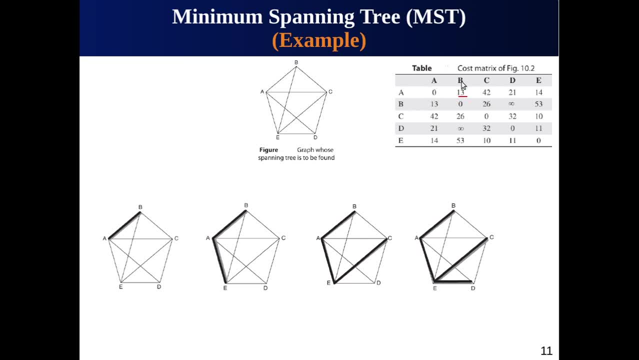 from uh from 8, sorry from a to b and then from from b to a is also here. it is from b to a. the distance is also 13.. because this graph has no directions, it's not a directed graph, so the distance is same from a to b and from b to a, from either side. you will travel, you will have. 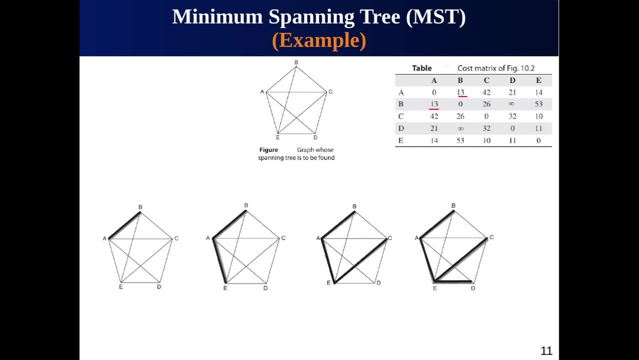 to travel the same distance. okay, and similarly, the distance for each and every pair of cities is mentioned in this table. you can also write these numbers on the edges like this: from a to b, we have 13.. from a to c, we have 42.. 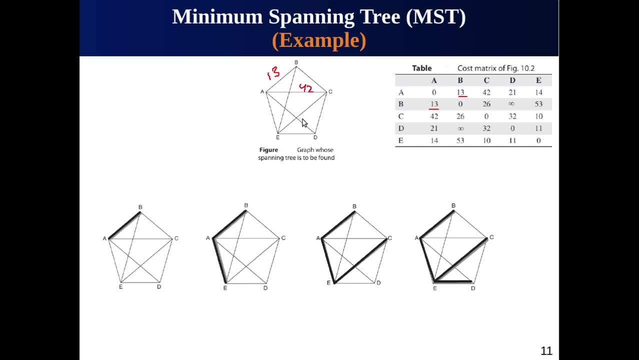 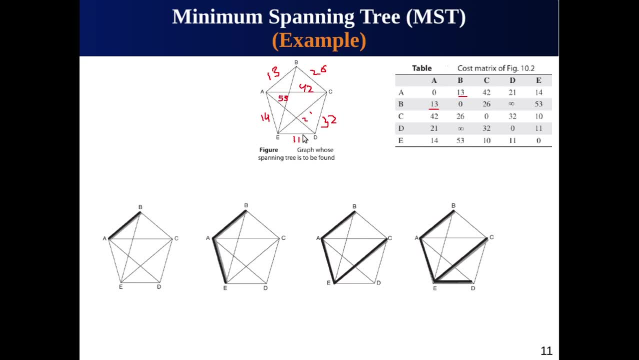 and if i left someone, you can write them as well. now our our task is to find the minimum cost to travel, for example, from a to e. in order to form a spanning tree for this graph, we have to take a distance which we can find from the source node. for example, our source source node is a. 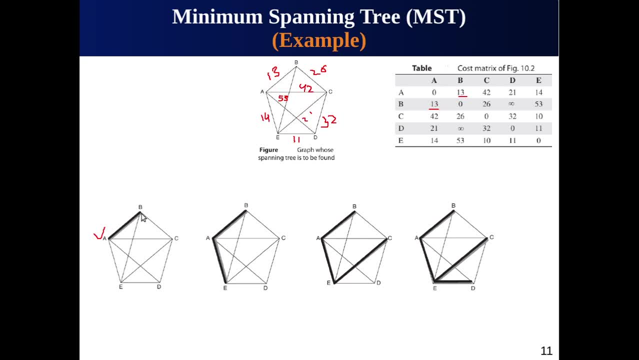 and then from here we have to find the distance to all the adjacent, to all the adjacent. not all the adjacent, but the more feasible, the more the link with less cost. so if you consider: from a you can move to b, you can move to c, you can move to d and also you can move to e. 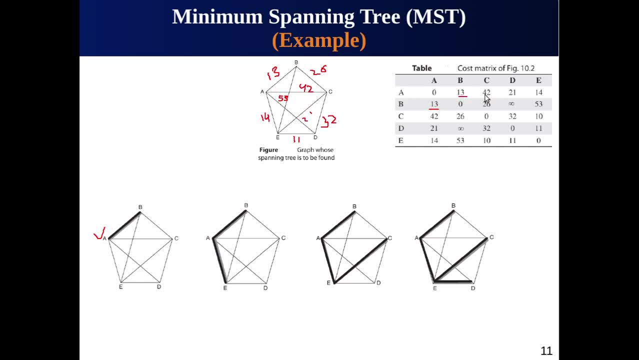 let's see here: from a, the cost to b is 13, 42 to d is 21. to e is 14. what is the less cost in this row? it is 13 and it leads to b. so we have selected this arc or this edge. 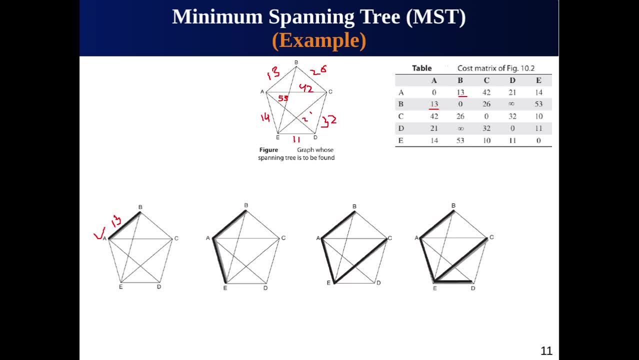 as per the values given in this table, the minimum cost edge is from a to b, or you can say from vertex a to vertex b, and the h a b is therefore selected in the first iteration and it is shown in the figure, and these vertices that we have selected would be: term is active, so a b link. 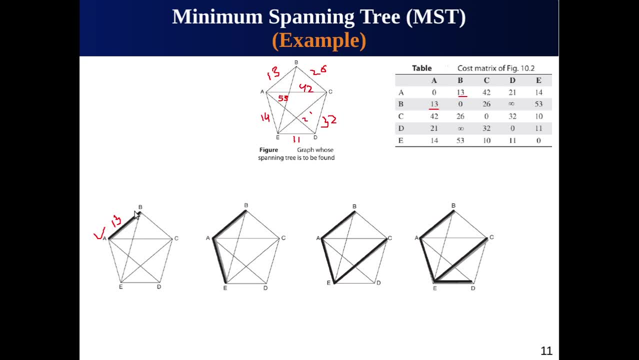 is now active, or vertex is vertex a and vertex b. they are now the active vertices and this is followed by selecting the minimum cost edge from b to a. let us see: from b to a we have 13 and others are very much large number, so we have to select it as well. from b to a is also the same. now the edges, uh date, are: 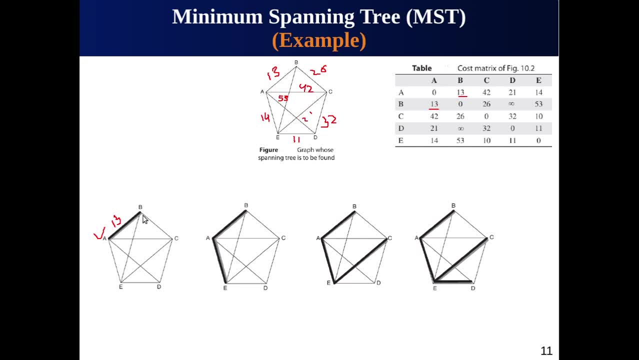 adjacent to the active vertices a and b. they are a, c, a, d, b, c, uh, e, e, and then we have e, c and e d. all these vertices, or these links, are adjacent vertex b and e, which are the active vertex now, but the minimum cost edge among all these. 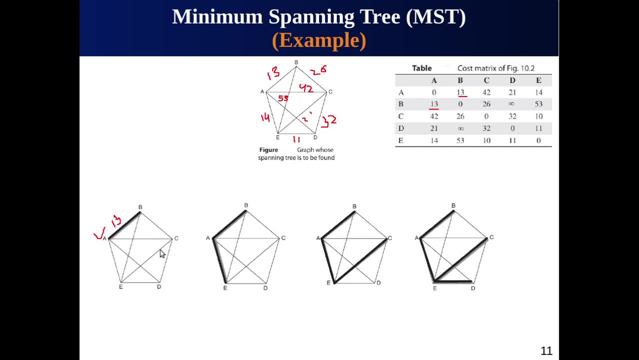 vertices. we have selected edges. there is ec. you can see it from the table that the ec is actually have less cost in all the available options, so we will select this edge. that is sorry, not, uh, not easy. let us revise the con. we have the vertices which are actives: a and b. 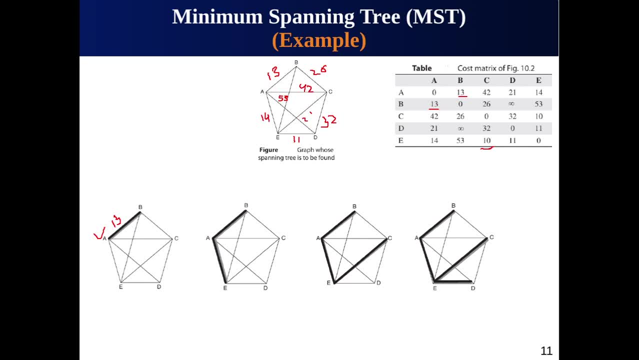 okay, now they are active. well, and as you can see that the adjacent vertices from a are: aые cost is 42, aee, the cost is 14 and b the cost is 21 and, similarly to b, there is be, which is 53, br pend spot, which is 53, and a isg, which is 16 plus. so we can also 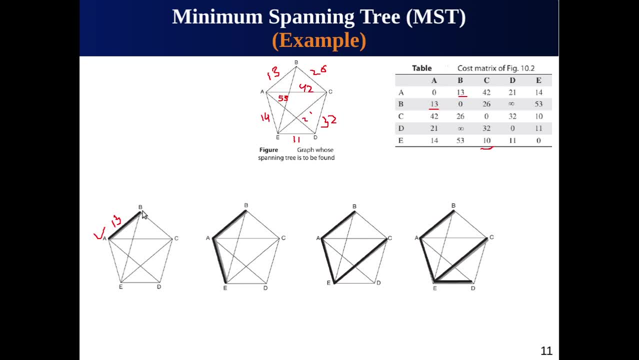 bc, which is 26, and that's it. among these, the smallest cost is for a to e. as we can see, the cost is 14, so we will select a, e as well. now, this is the case. now we have active vertices a, b and c, we have to repeat the same process. the edges date are adjacent to the active vertices a, b and c. 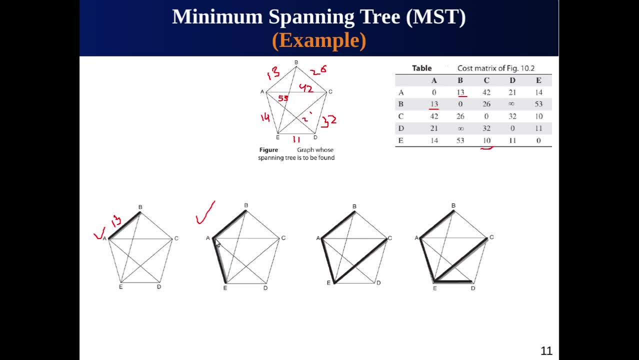 we have to identify them and they are: from a, the adjacent are ac and at. from b, the adjacent are bc, b, e. from e, the adjacents are e, t and e t. now you have to find the minimum cost edge among these edges and after looking at the table, we come to know that the, the the smallest weighted. 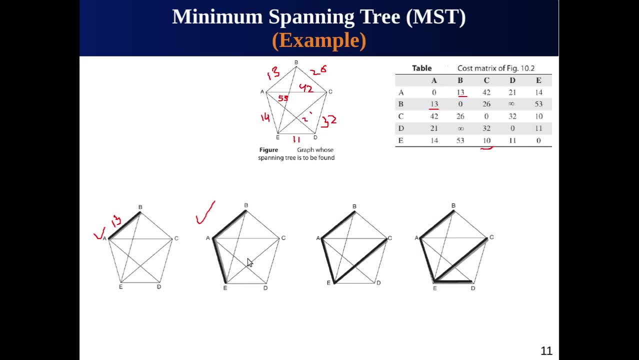 edge is from e to c, having the value 10. so we have to select this and then now we have to move one step forward. now the active nodes are a, b, b and e and the adjacent edges are which are not yet selected. they are ac and also ad. from b, we have b, c and 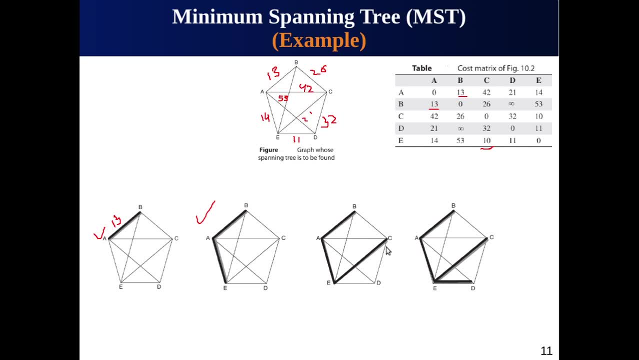 b, e and similarly, from d we have d, c and from e we have ad. and now you have to select the minimum cost among these unselected edges. after looking at the table, we came to know that the smallest one among them is from e to d, and there is 11, so we have selected. 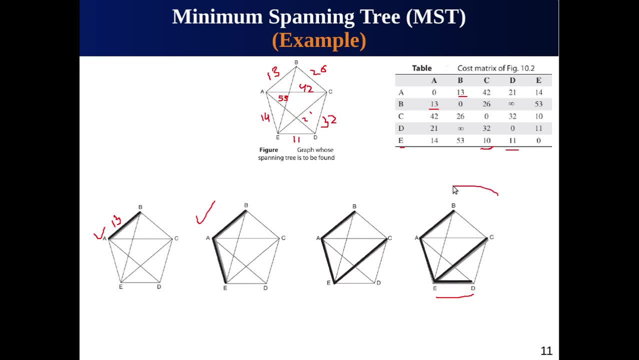 it. now. that's it. since all the vertices, if you see here, have been covered, the task is now accomplished. okay, you see all the vertices, all the nodes are selected and now we have to select the minimum cost edge among these three images and we have to start. t is soap analyst, so we have accepted here. 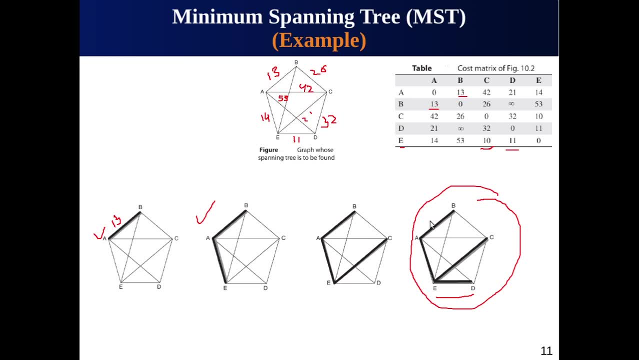 and we have inside added one default value. one default value. then fill in the 해야. I mean what? what? one default value if I use ha, it's gonna be negative. so let's skip this set excepted, so we can use our default value and you can also alter the number of edges. and order the value care, if you choose to call it, byальным flavors, by what you would do if you are not familiar with bootwork. also, we can double click, pay no, which is even more complicated. this has become a 1-2, also important because we have to do this. first of all, we have in the our were looking for a minimum cost edge. we have to start with identity set up. 1, 1, 3, 4, so i call it pin 1 again. this is the initial and also i white and we can see here that we have two dots there in section 7th or ruling point number 1, and of course we want to 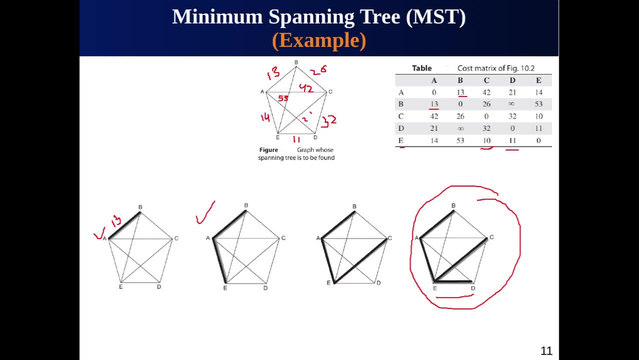 we have four vertices, sorry, four edges, and four is actually, if you, if you calculate the number of vertices, there is five. so five minus one mean n minus one equal to four. there is a formula it fits okay. so this approach qualifies to be a gritty approach. remember, we are studying approaches. 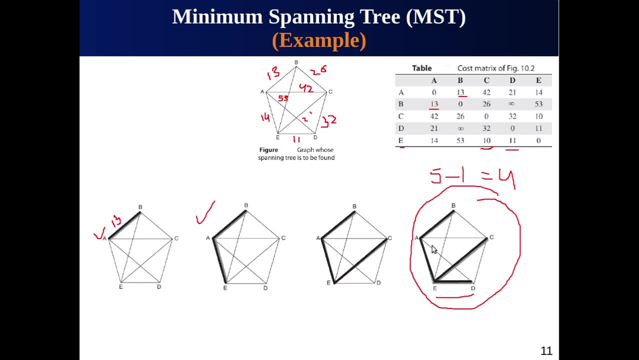 which actually follows the gritty optimization problem. and this is actually a gritty approach. why? because the decision is taken by considering the path which is the most promising. eight date, particular time. we are only looking at the next level, you, the next solution which is best at that time, at that particular time, at that point of time. 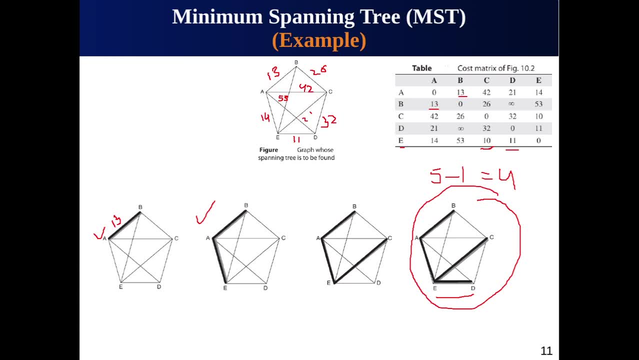 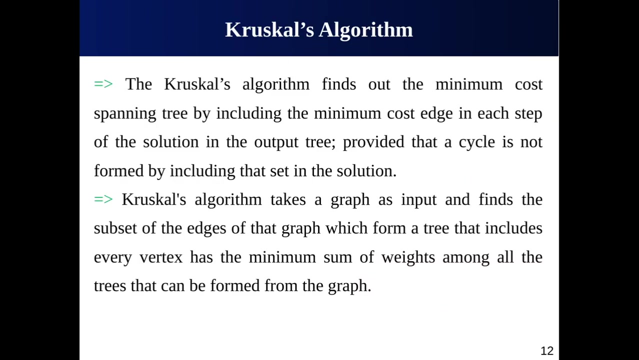 okay, so this is actually a gritty approach and this is best for many scenarios. now let us uh see how we can actually find this MST for a graph by using different standardized algorithm. we will focusing on two solutions. the first one, of date, is known as critical algorithm. let us see what is critical algorithm. 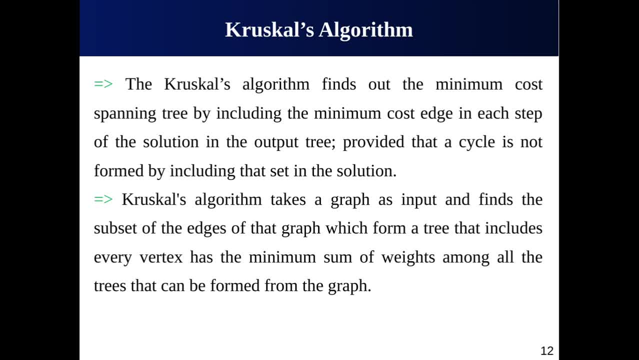 uh, the critical algorithm finds out the minimum cost spanning tree, or minimum spanning tree or MST, by including the minimum cost edge or the minimum cost link in each step of the solution and we have to put it into the output tree. the condition remain is the same: you have to proceed in such a way that you will have to avoid the cycle. cycle should not be performed. 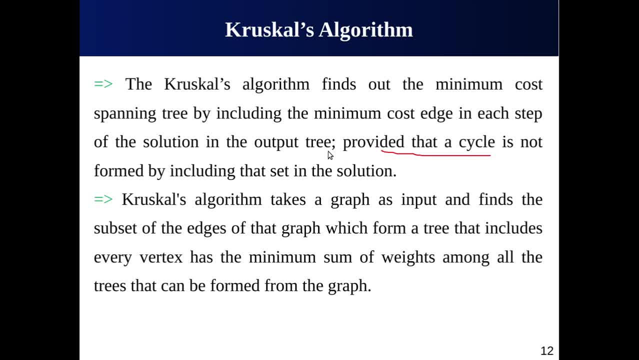 okay, the risk skill algorithm is actually a minimum spanning tree algorithm. it takes a graph as an input. remember, we have to provide an input and the input input is a graph. then, after providing the input, this algorithm will find the subset of the edges of the graph which actually forms a tree. 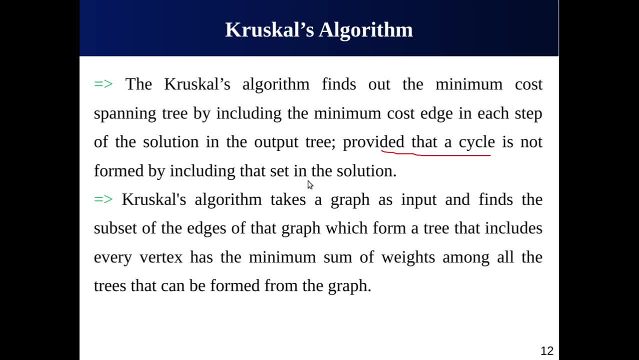 and the objective is that the resultant graph must have minimum sum weights. among all the possible solutions, some of the things that i have highlighted here. they are important to remember. first thing is that in the griskell algorithm, we have to give attention to the edges. to be more specific, we need to give attention to the cost of each edge. 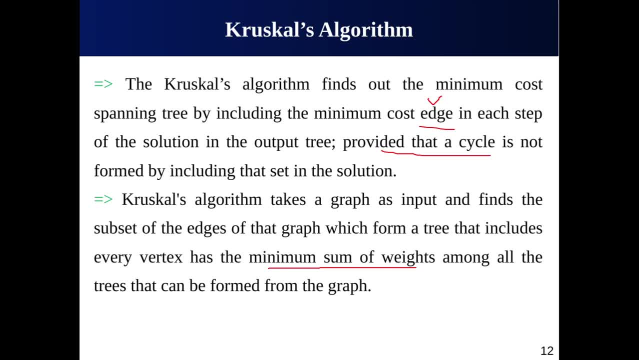 or to the weight of each edge or each link. that is important. second thing is that we have to proceed towards the final solution, but we need to avoid cycles. for example, if you are moving from a to d and there is a cycle in between before reaching to d, then you have to avoid that path. you have. 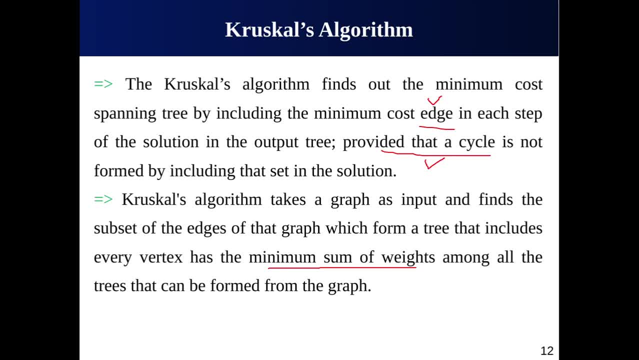 to avoid the cycle. we have to avoid the loops, we have to avoid the circuits. okay, and finally, uh, the algorithm actually identify the solution which will have the minimum sum of bets, mean the optimal solution, as we just saw here in this case. okay, so these are the objectives of the griskell algorithm. 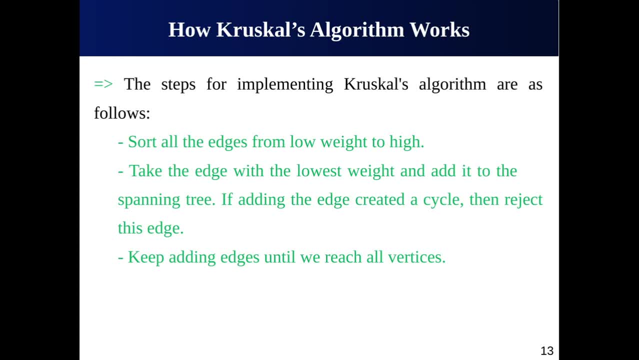 now let us see how it actually works. let me repeat, state: this algorithm risk actually falls under a class of algorithm which is known as greedy algorithm or greedy approach, and they find the optimal solution at a particular instance of time with the hope that at the end we will have an uh, a solution that is going to be global, like, for example, if something is good. 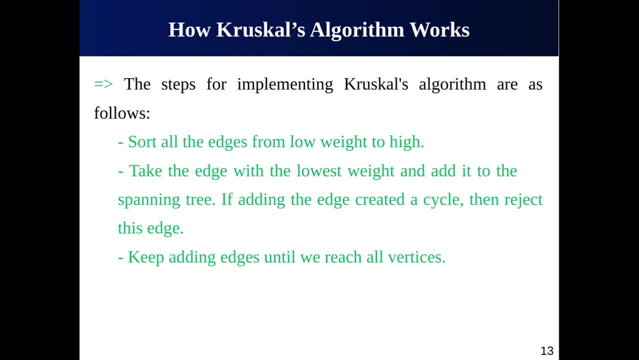 for this particular case. at the end we will get a solution that will be optimal for for the global problem solution is going to be optimal for every um solution that is going to be optimal for every, for for the big problem as well. okay, so we start from the edges. remember again: we start from the. 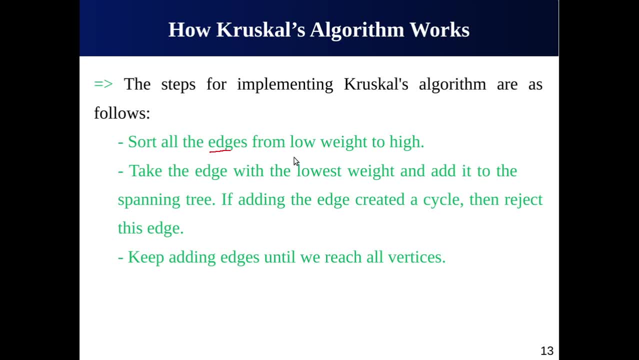 edges. and then, first, we have to sort the edges in ascending order from low weight to high weight. okay, let me tell you one thing: these steps are only for implementation of this algorithm, but our concentration in this course is not on the implementation. okay, so we will not go into the 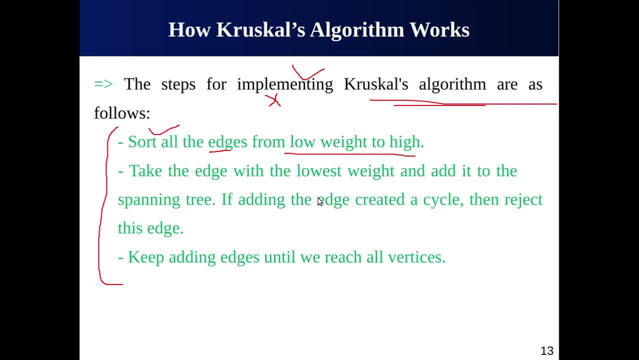 further details of the implementation concepts. rather, we will focus on the algorithm, its operation or how it works by taking some examples. but still, you need to know that if you want to implement this algorithm, the criteria is that you have to start the edges in ascending order from low to high weights. after that, in the second step, you will have to 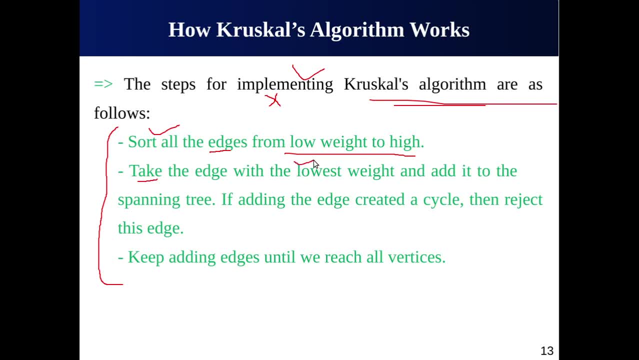 take the edges, it has the lowest weight and you will add it to the spanning tree or the output. but remember, if date solution lead to a cycle, then you have to reject it. you will not include it into the output. okay, because we will try to avoid cycles, the loops, and then you have 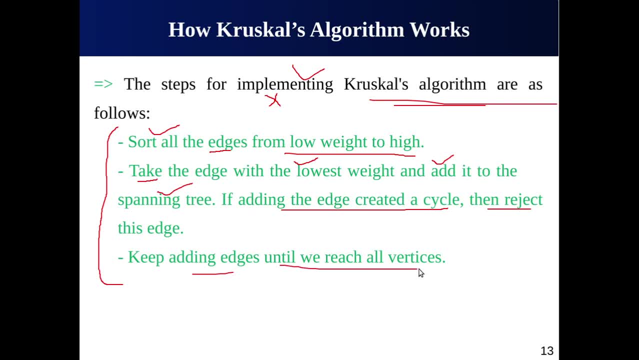 to continue repeating the step, adding the edges, until we have covered all the vertices, until the graph is connected, fully connected, all the vertices are accessible. if we reach this condition, then it's time to stop. this is how we can actually implement risky algorithm. now let us see how it actually works with the help of an example. 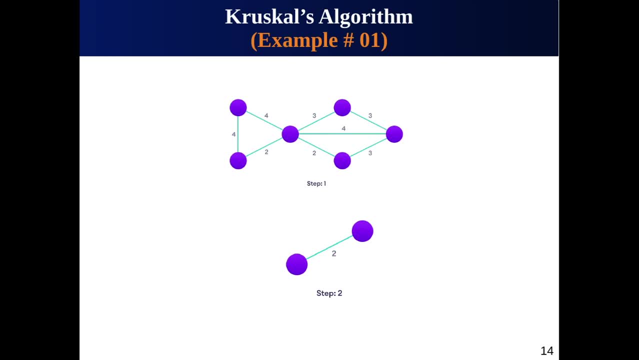 example number one actually is about grvania algorithm and how it works. the graph which is mentioned here- that mentioned here- is actually a weighted graph. it required a weighted graph in order to decide which solution is optimal and also the graph has no directions. undirected graph. 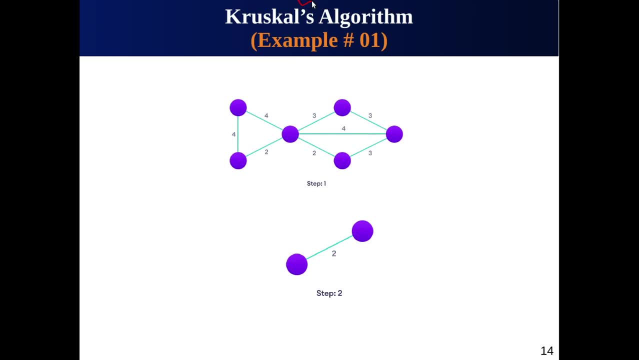 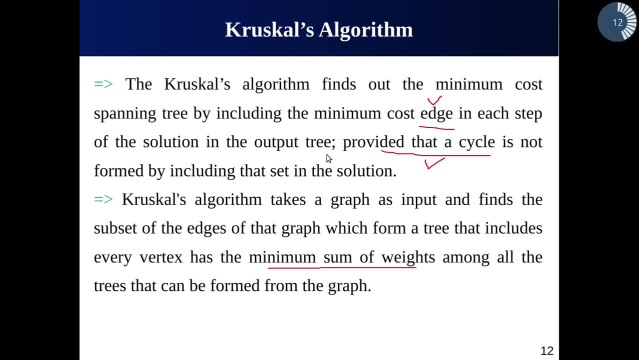 step number one of the Criskell algorithm is, let me stress here again, we have to stress the edges here. later on I will compare Criskell Algorithm with the Graham Algorithm, but there it is important to note that here we are actually focusing, concentrating on the 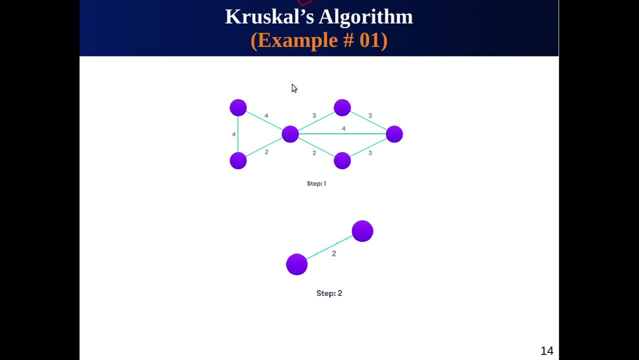 edges, but we have to start from the Edge, which as the least weight you can see. every edge has a cost associated with it. what is the lowest number here? what is the lowest cost here? what is the lowest cost? cost the data, the cost associated with it. data, the value generated, level. 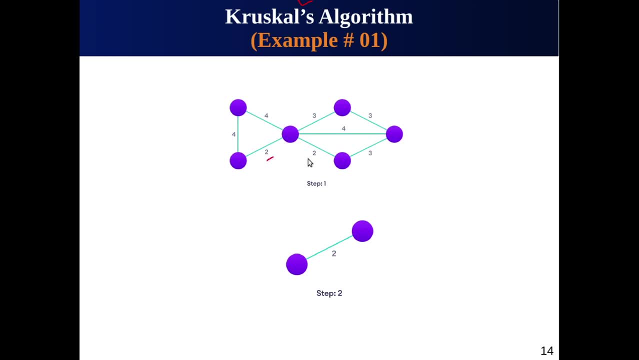 weight. here, that is two, but wait a minute. we have two edges with the same weight. now what to do? which one to select? okay, there is understood that we have to select an edge with the least weight, but if there are more than one edges with the same weight, then what to do? which one to choose? 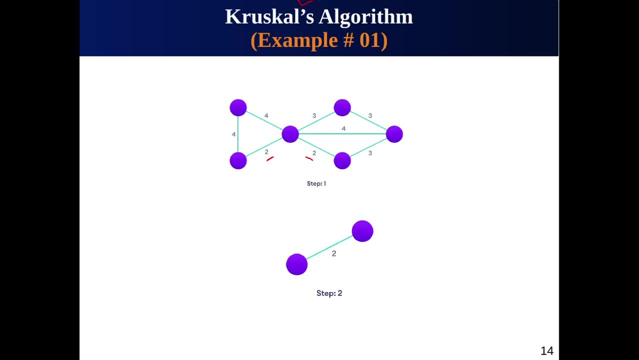 option is your choice is your. you can choose any one of it. you can choose this one. sorry, the nodes are not level so it will be a bit difficult to to name it properly. but let us see a and this is node to B and this is not C. so you can either select A to B or you can select B to C. cause the: 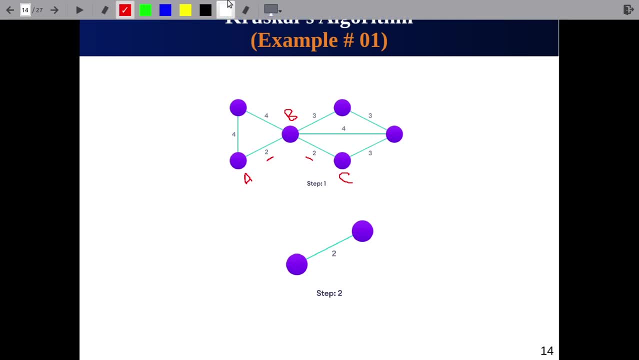 weight of these two edges is the same and select either one. we are going to select this edge now. after selecting this one, the next step is to choose the next shortest edge and add it to the output, our output, for the time being. so the next one is this one is to: 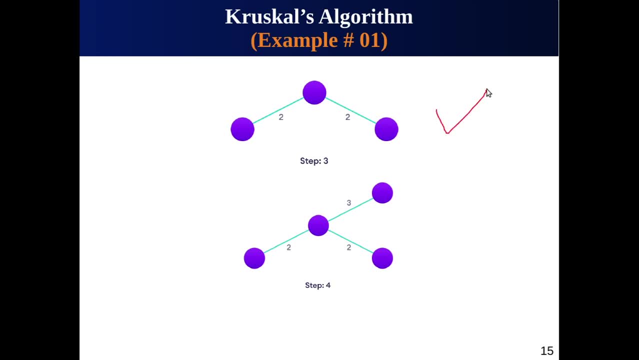 edit output. that's it now. we have selected these, the vertices and two edges. what next? repeat the same, choose the next shortest edge. it doesn't create a cycle, remember the condition. and then we have to add it here. so the next possible edges is edges, are this one? let's suppose is, and we 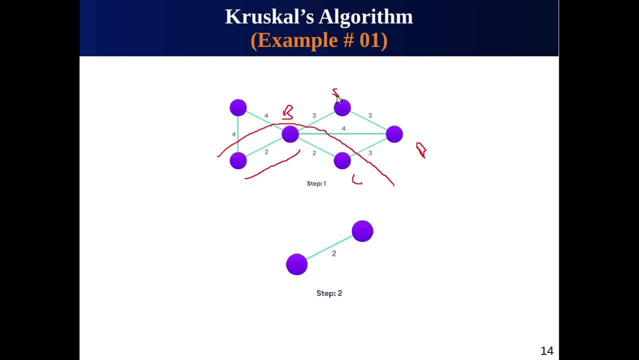 he which one we have to choose. either C to D or B was. both have the same, are the same weight. let's suppose I have to this one now. vision is like this: it has been selected, has been selected as well, for the graph is like this again: choose the next short test age date does not create a cycle and add it. 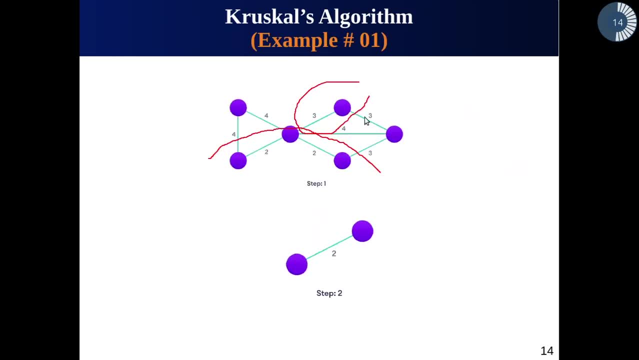 to the output. let us see what is going to be the next one. okay, here you can actually watch it. we have again two edges with the same number three, so let us this one bring the weight free and add it to the output. yeah, they have selected this one. 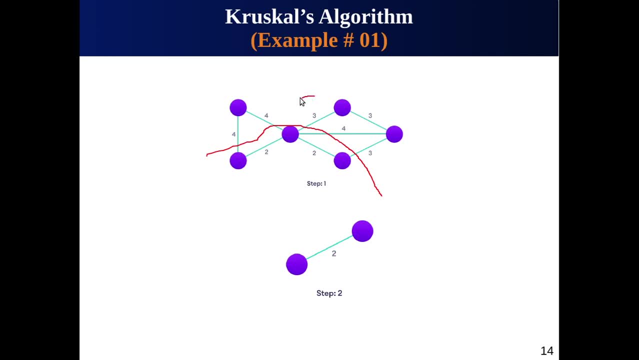 but the situation is going to be like this: already selected, already selected. we have to select either this or this. so they have selected this one already selected. and the situation is like this: yeah, I want days. I want two colored edges for the last one. we have two selected. what do we do now? 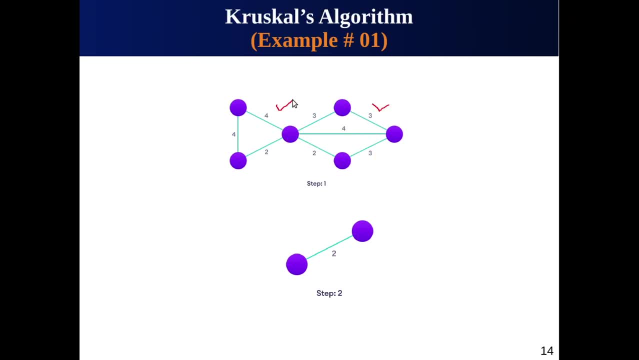 we have to select either this one or this one. we can remove the first and second angle so we can skip this one and the this he likes it or this one. but we cannot select this. why? because it will create a cycle and we have to avoid the 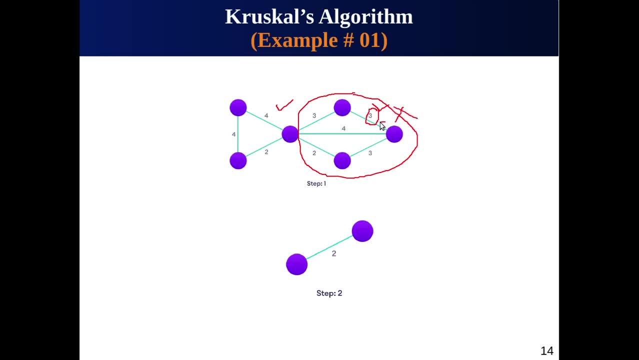 cycle. what next? ignore this one, although it is less, although it is the minimum value available at the moment, but we have to choose four. so the next step is like this: select this. it will create a. create a cycle. now, at the end, you will see that we are done. 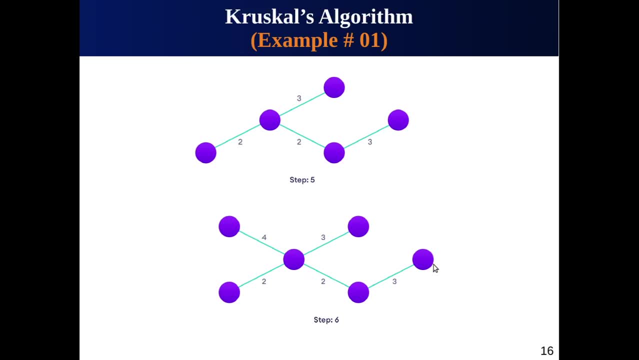 all the vertices are now connected and we do not have any cycle here. and this is how we use criskell algorithm: find the mst. and this is actually a minimum spanning tree because it has the minimum cost. and this is actually a greedy approach, because we select. 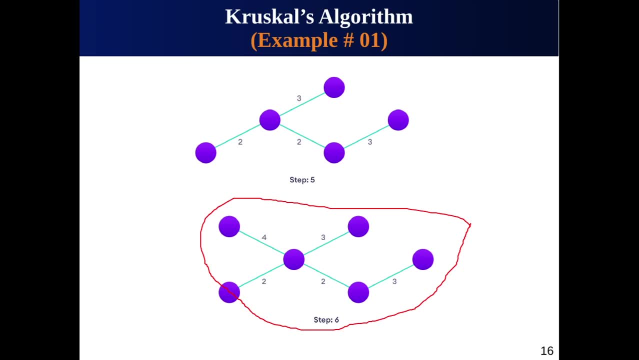 the solution which is best at that particular instance and we, we we assure that the global solution, the overall solution, is also the optimal. but there is not not true in always, in all the cases, but majority of the time we will get a globally optimal solution, as well as the result of Criskell. 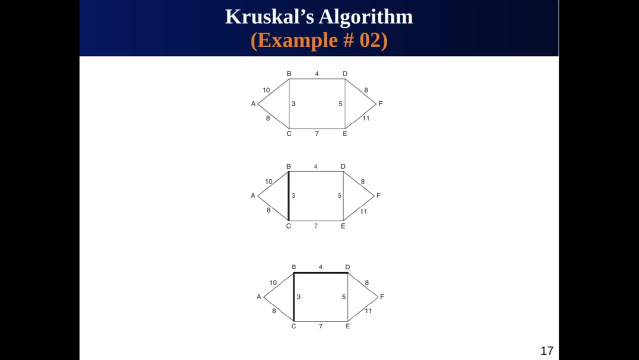 let us consider another example of the Criskell algorithm. here we have to use the same algorithm, the Criskell algorithm, for the graph which is given here. now we have the vertices numbered from a and again they are connected by links and the links every link has a number has a weight associated with it. 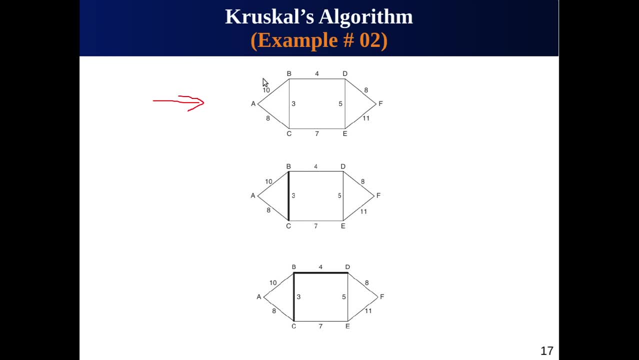 which actually represent the cost or page or value, which is an arbitrary number. first thing, first remember: we have to focus on the edges, we have to start with the edges and then we have to start with the edges and then we have to start from the edge which has the lowest value in this graph. let us see, let us. 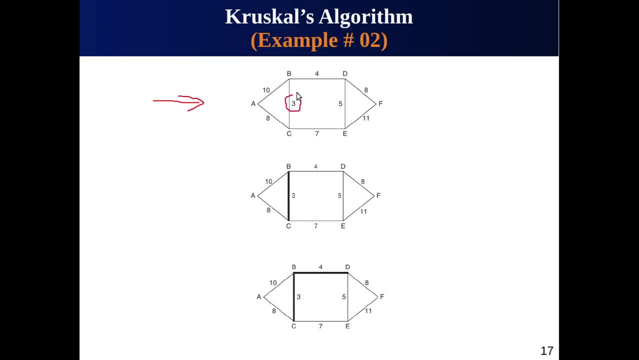 find: okay, we got one. the minimum cost is B to C. since B to C is the least cost edge, then B to C will be selected. the dark line means that B to C has been selected in the first iteration of the Criskell algorithm. what next? 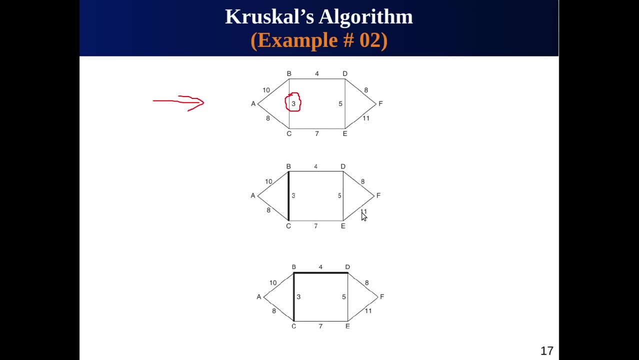 now, from amongst the remaining edges which are not dark, we have to select the least cost edge. let us see. but they must be, must be reachable from the, from the active nodes B to A, 10, B to A, 8, B to E7, B to D, 4, I think the least cost is, and there is B to D, so make it Dark. B to D. 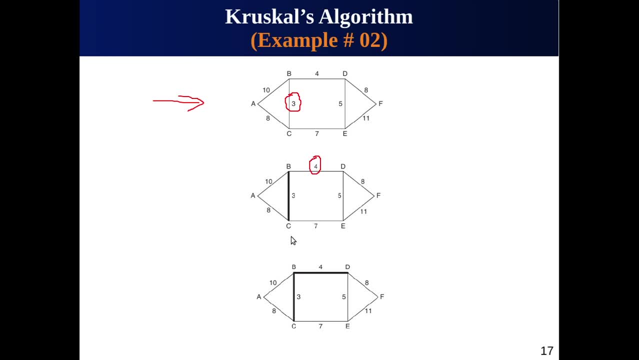 B to D, 4, I think the least cost is. and there is B to D, so make it Dark. B to D, so make it Dark. B to D. now the active, the active uh nodes are b? e. now, from amongst the left over edges, uh, we have to find the one which is the least. 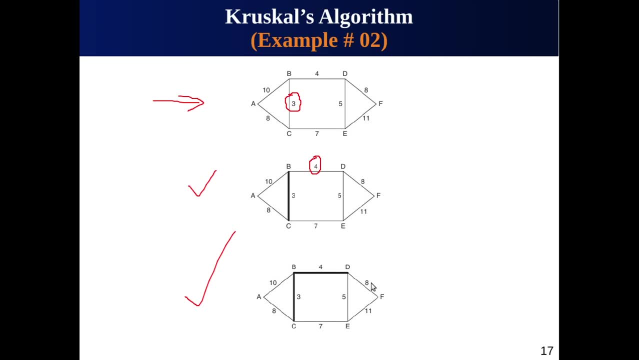 which has the least cost. so, if you pay attention, the cost here is seven, here we have eight, five, four is already been selected, ten and eight- i think the least cost is five and that has been selected and put into the output file. repeat the same process. find the minimum cost as you. 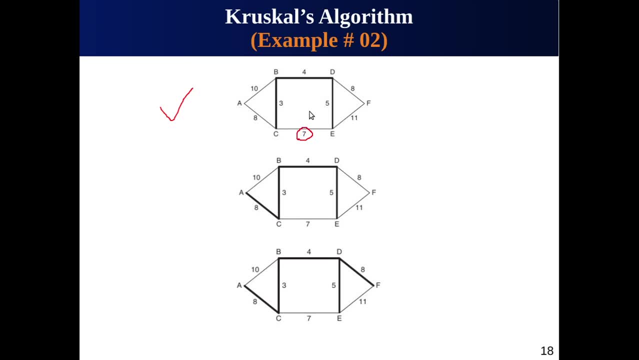 can see, the minimum cost is seven. but we cannot do it. we cannot select c, e, h, i. if you do this, it will become a cycle. see, this is the cycle and we have to avoid the cycles. so we cannot do it, we have to search for something else. a number there is greater than seven, so the edges. 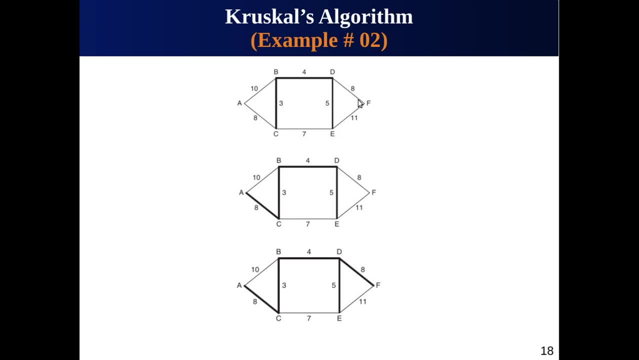 if you pay attention, here we have eight. here we have eight from a to c or c to a, and from a, d to f or f? e. we have the equal weight, that is eight. so you can select any one of them. let's suppose we have selected a to c. 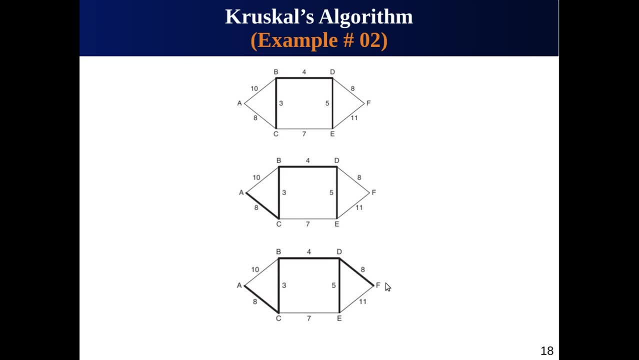 that's it. in the next iteration, we will select d to f and that's it. after after this. uh, you would see that now all the vertices are connected. for example, i want to travel from a to f, is it possible? yes, go to c, then to b, then to d. yes, that's it. 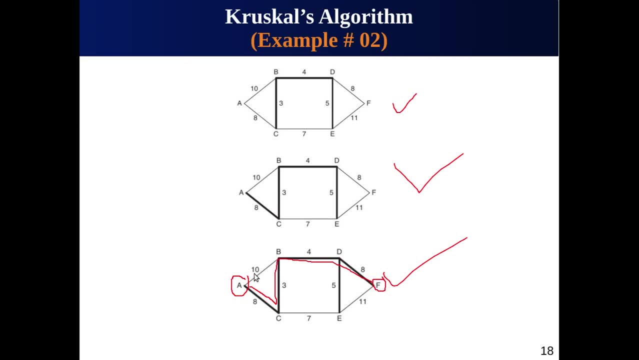 and get involved with the cycle. if we want to pumpkin sap these, we can do it easily just in here. we'll go to to c and we will go to the объ of erhalten amongst and: uh, this is the right order right here and it doesn't matter. 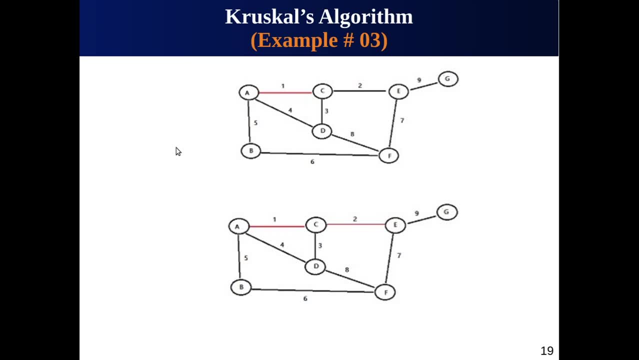 좁, not that easy to duplicate here and it doesn't matter. we can do anything herewith. we can написe this and we can pick the right parameters to fit here as the graph larger. this is actually a minimum spanning tree, which is a gritty approach, and we find this minimum spanning tree by using the grayscale nationale, gradually, i'm so you first have to add the cost of the individual edges to get the overall sum. this is actually a minimum spanning tree, which is a gritty approach, and we find this minimum spanning tree by using the critical algorithm. finally, let us see a third example. i would rather say that you could try this example by yourself. only two steps are mentioned here. first, you have to give concentration to the ag Christian team. 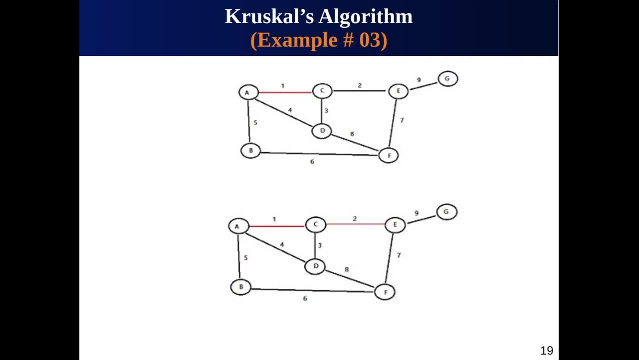 to give concentration to the edge, the numbers associated with each edge. the lowest number is one. so mark these edge as red. now these two nodes or vertices are now active. see the neighbors, see the directly connected neighbors. to b, the cost is five. to d, the cost is four. to d, the cost is: 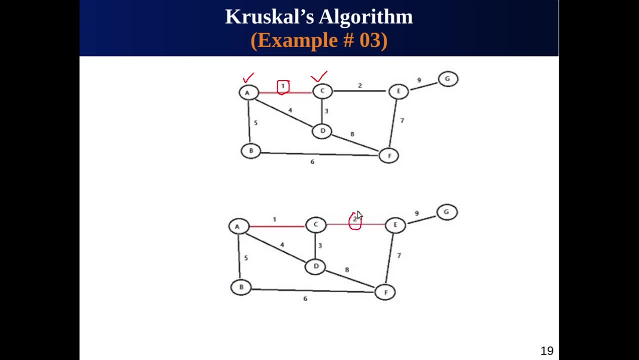 three and to e the cost is two. i think this is going to be the next choice, because there is now the minimum value edge in the remaining, and then you can proceed with the rest of the graph. finally, you will get something like this: there is a minimum spanning tree, the edges that are highlighted by 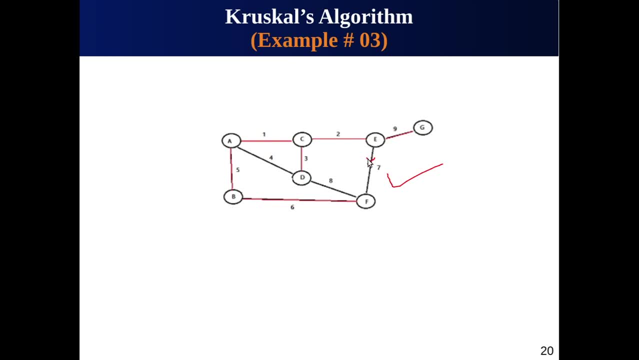 the red, they are actually considered and the edges: they are not highlighted, they are not considered, they are actually ignored. now we have a fully connected graph, undirected graph, and they, the edges selected, are actually the the minimum cost available at that particular time, and this is a greedy approach. 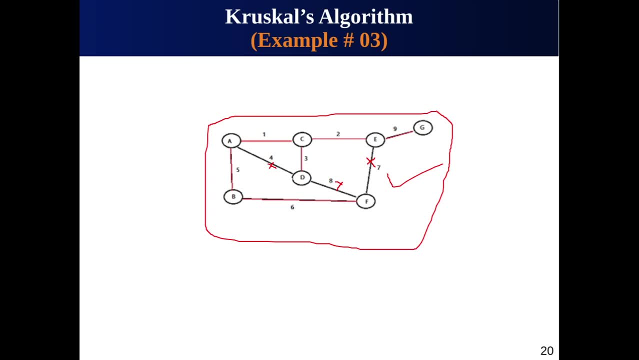 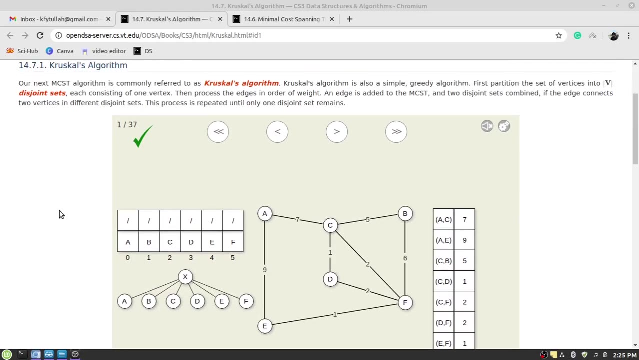 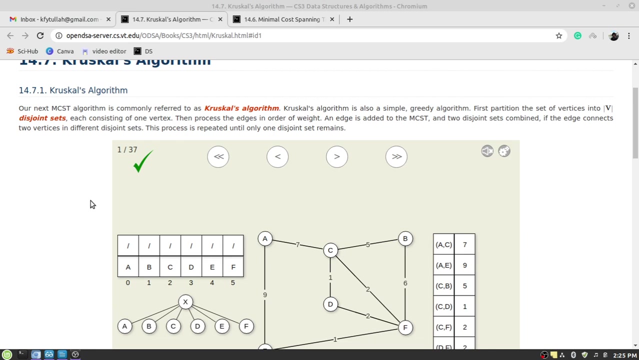 okay, guys, uh, before moving to the next algorithm, i would like to do an animation. please give me time. okay, guys? uh, here we do have a an animation of the critical algorithm. this is something related with the implementation, but we will not go into the details of the implementation because 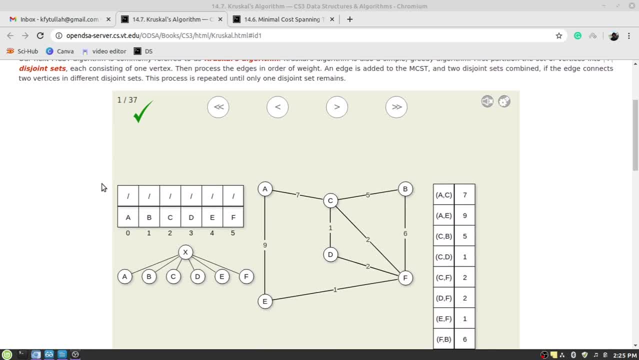 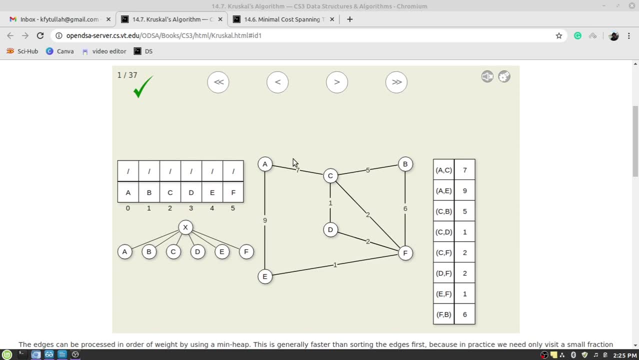 they have used the implementation of the implementation of the implementation of the entertainment of the implementation of the implementation of the implementation, in order to facilitate the implementation. we will focus on how the actually the crystal algorithm technique work. let us start. we have a graph given and indoor, 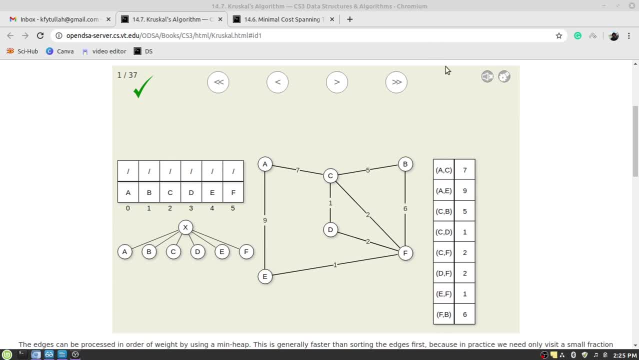 remember, for the implementation. uh, you have to write the, the edges, along with their values, their cost, their weights, mentioned here, for example: a to c, we have seven. a to e, we have nine, and other as well. and here we have the division ofância football, the disjoint cells, the disjoint set, and this is actually the tree. we have all the nodes mentioned. 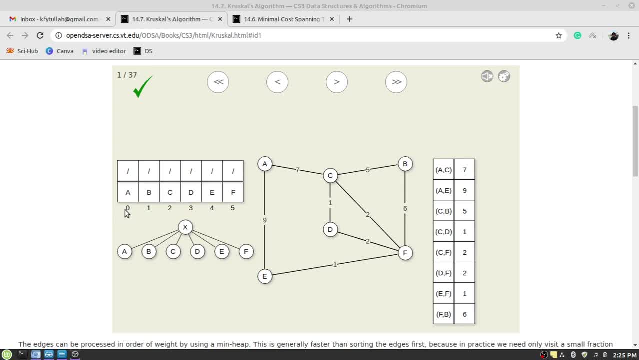 here. this is actually an array. starting index is started from zero, but we will not go into the details of here. let us focus on the classical algorithm itself. let us start, okay, processing edge EF. why? because that is the least value. the least value of the edge is from E to F. so we 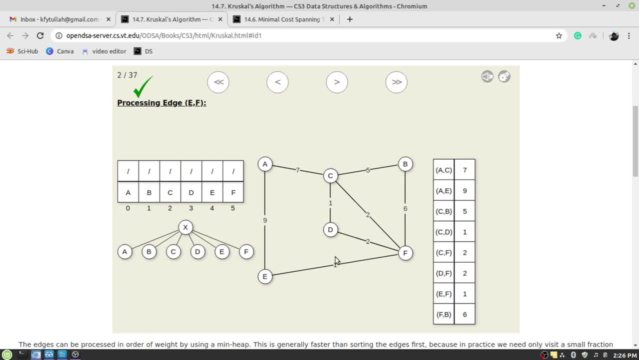 have selected this edge. let us move one step forward. okay, here is something related with implementation. both the nodes are considered. they are E and F. E has. no, uh, the parent of e is actually e. this is not a parent x. okay, the parent of e is e and the parent of f is also f. 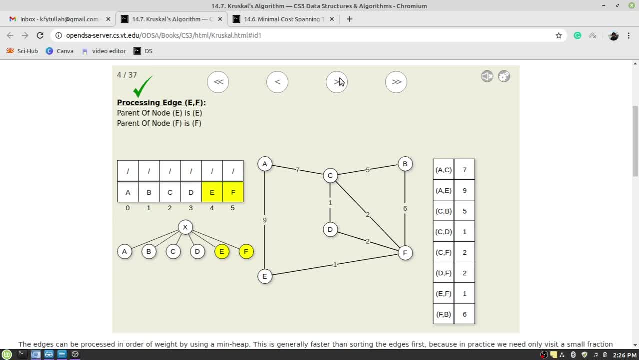 so we need them to build a relationship and there is going to be like a union of the nodes. now, e, f, we have a path and the cost here is one we have to concentrate. here we have identified the edge with the least value, that is, from e to f, and we have give, give it the red color, which mean okay. 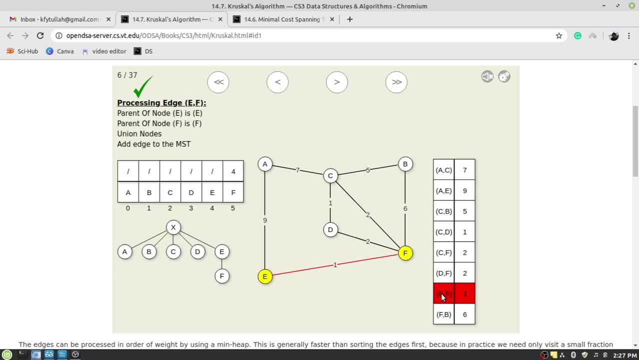 now, this has been part of our solution. if you want to travel from e to f, that is the best route. next one: identify the second path between two vertices with the minimum cost or value or weight. here we have nine, here we have seven, we have, we have two and we have two. oh, 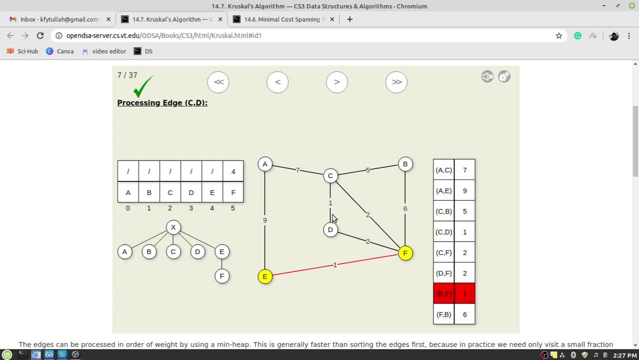 two paths with the same, uh, with the same value. up to you the one which either one you will select is: we have selected c to d. sorry, sorry, sorry, sorry. we have another um value. there is one, there is less. okay, so we select it from c to d. now see the parent of c itself and the parent of d. 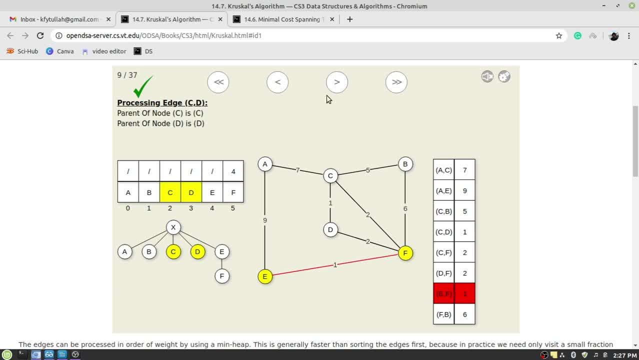 is d itself. we have to re-union them. e will now be the child of c, that's it. but we are not interested in this. we are interested here. we have identified the next edge with minimum value and that is c and d. so it will be highlighted. that is part of this. 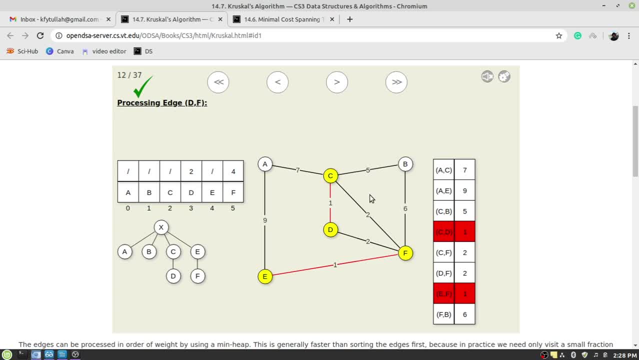 now next, find the next edge with the minimum value. that is, either uh c to f or or d to f, or you can say f to c or f to d, up to you. either one you can select. we have selected from d. have selected from d to f, this one, okay. 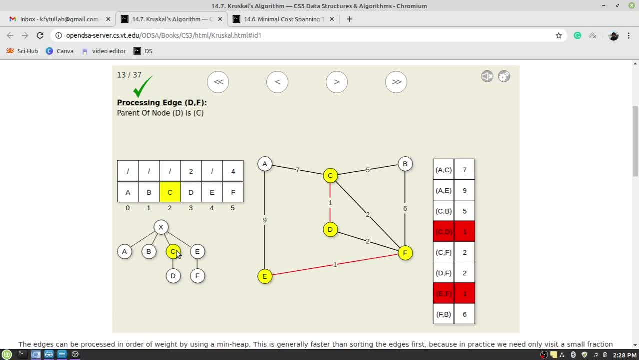 now see, d has a parent that is c and also f has a parent that is e. so what does it mean? means that i have to union them like this: and f is a parent, because the parent, if you see, uh, the parent of b is c and the parent of f is e, so we can. 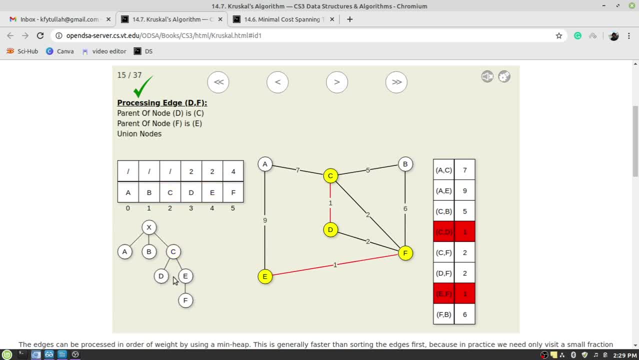 reunion them like this. now, the parent of b and e is, but here, uh, we have to uh to color them red like this. and this is now our path from d to f, and this is part of the output. next, this is important now, look, uh, the minimum value is two and the node, the edge, is from e to f. 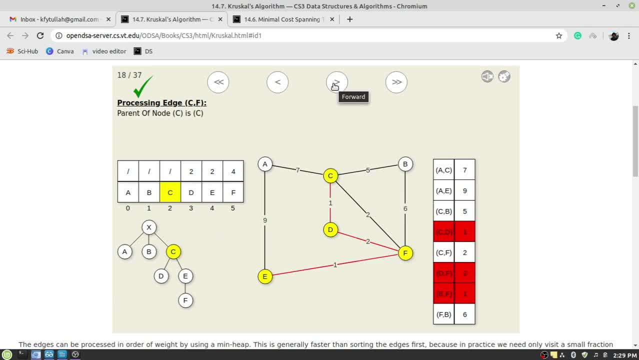 now see: what is the parent of c is the parent of of c itself. now, what is the parent of f? the parent of f is c as well. what does it mean they, if they have the same parent? it means they are already union. okay, so we cannot reunion them. and if now you see here that is not possible from c to f, why? because 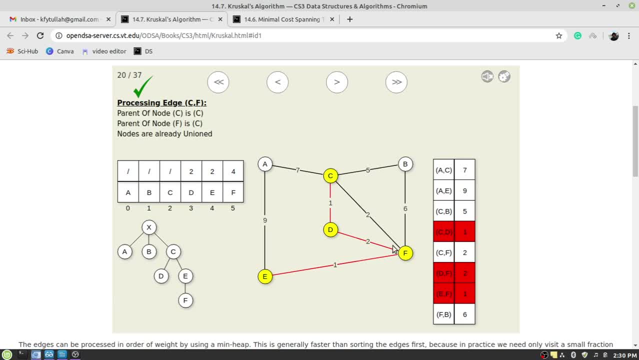 if you make it part of the output, part of the solution, then it will become a loop and that is not possible. we have to avoid the loops, and you can see from here as well: that is not possible. we will not make it part of the solution, we will ignore. 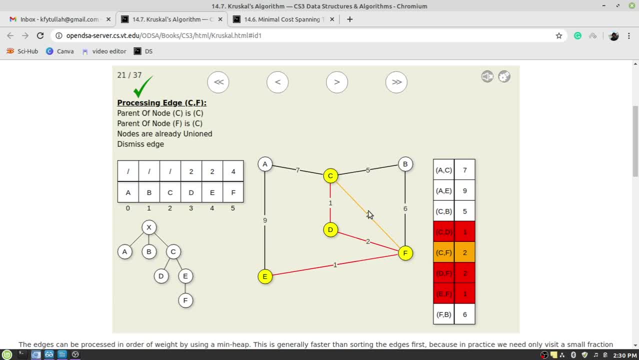 this edge, although it has the lowest value now, but we will ignore it. next, find number at the edge with the minimum number, and that is five. the nodes are c to b. let us see here: the parent of c is c itself, okay, but the parent of b is b itself. 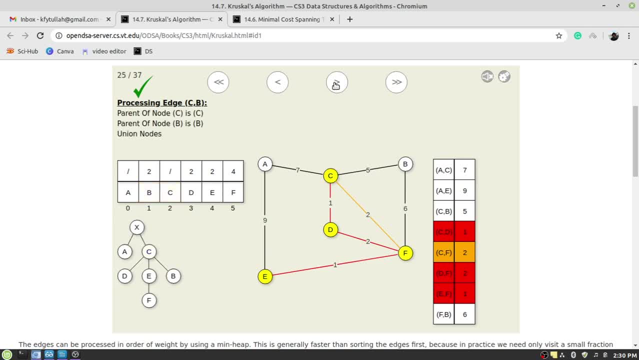 so c will become the child, sorry, b will become the child of c. now, okay, concentration should be here on the, on the on the graph e to b. the cost is 5 and it does not lead to any uh, to any cycle. so we will identify it and we'll make it part of the solution. 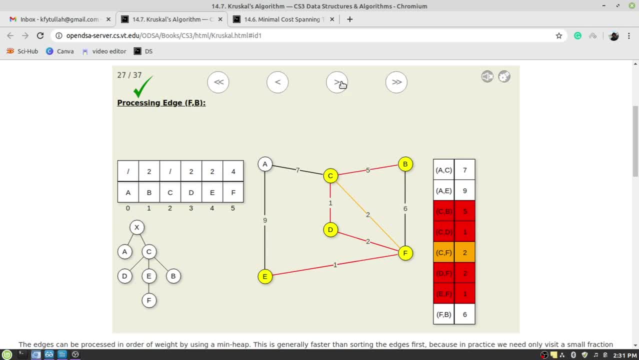 next find the edge with minimum cost. it's seven, nine and six. oh, this has the minimum cost. so we will have to make it as part of the solution. not part of the solution, but we have to consider it. let us see parent of c itself. sorry, parent of not c. parent of f is, you can see from here, parent of f. 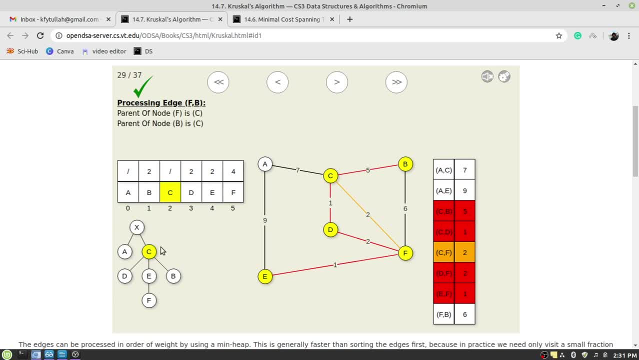 parent of b is always c. also, c means they are already in union, so you cannot reunion them. or if you see here b and f, you cannot join them. you cannot consider it to be part of the solution. why? because if you do it, it this line will become red, which means cycle, and we have to avoid the cycles, ignore it. 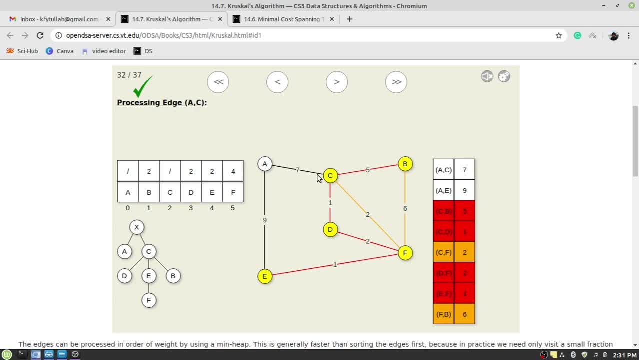 move forward. identify the next edge. with the minimum value. there is c to a where there is seven. okay, i will go for uh fast. now we will make it part of this. that's it. next, we left with a to e, but we cannot do it because it will become a cycle. that's it. 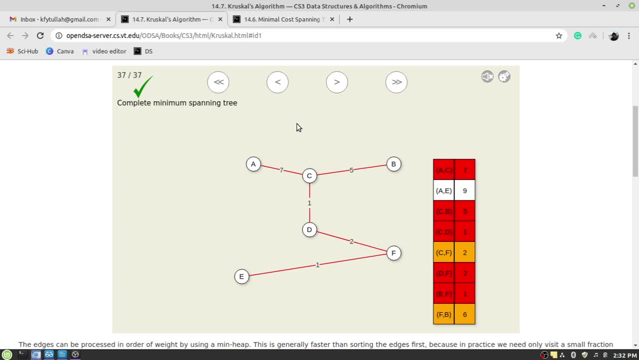 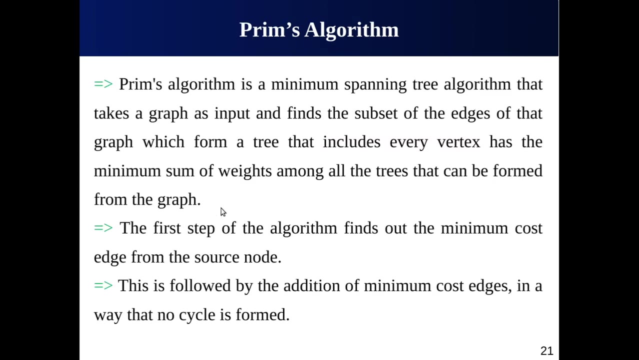 so this is the minimum spanning tree using crsql algorithm. this was an animation, you can try as well. back to the lecture. our second algorithm is known as prim algorithm. it is also a way, a method by using which we can find an mst or minimum spanning tree. 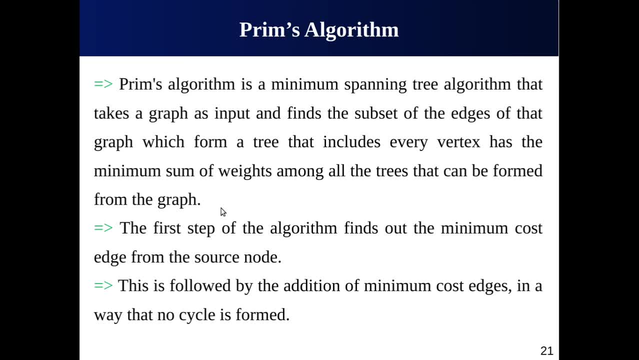 of course, not just any tree, but evenム the more freedom which is used to compute individuals. actually, the prime algorithm is simpler as compared to the crsql algorithm, and the prim algorithm is a minimum spanning tree algorithm that takes a graph as an input. remember, in both the cases we have to take a graph as an input and then we have to find the subset. 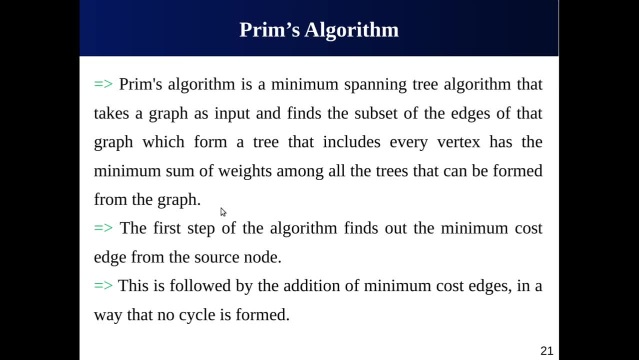 of the edges for that graph, which will actually form a tree that include every vertex. every vertex will have a minimum sum of weights among all the tree will be no cycle. so the first step of this algorithm is to find out the minimum cost edge from the source node. okay, uh, one thing i would like to say is that in prim algorithm we have to 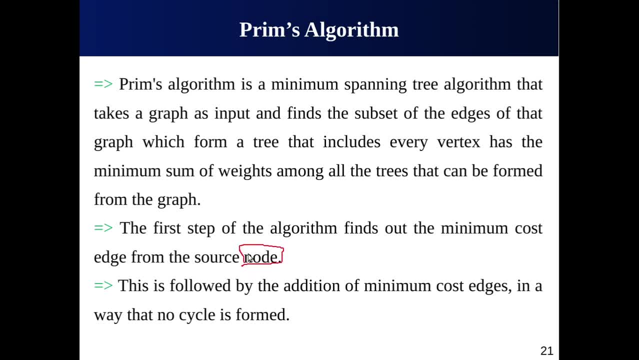 focus the node. remember, in the grayscale algorithm we were focusing on the edges, the minimum edge, but here we have to focus on the initial node, what is going to be the initial node to start our algorithm, separation of our algorithm. so the first step of the algorithm is to find out the 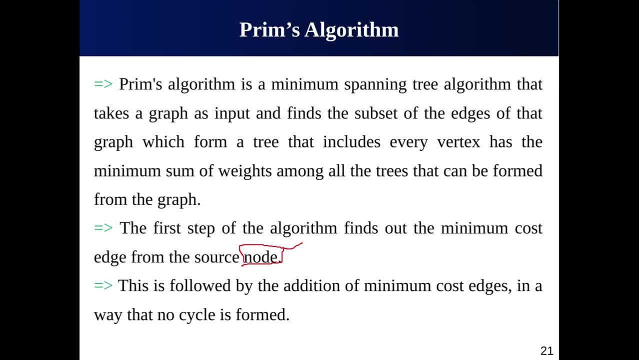 minimum cost edge from the source node, node, node. you do not have to pay attention to the edges in the first step. you have to select any source node and then find the minimum, the minimum cost edge from the source node. so, in summary, you have to give attention. 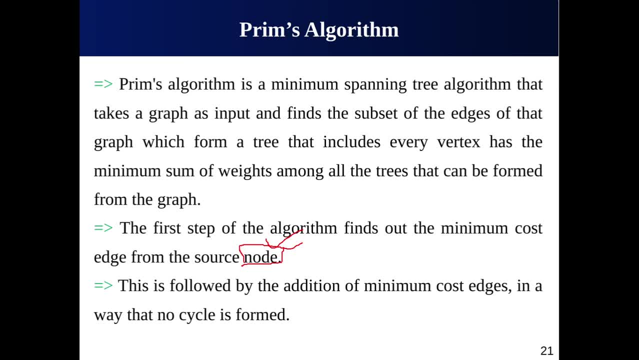 to us what is going to be the starting node for the algorithm to operate, and then this is followed by adding, by addition of the minimum cost edges. obviously, we have to do that in a way that no cycles are formed now how this algorithm works. this is something again related with the implementation. 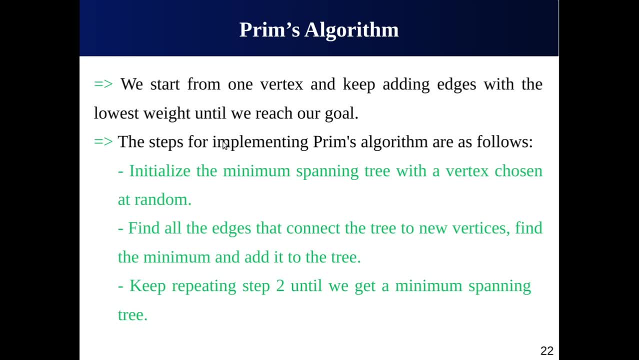 but for understanding, let us see how it works. actually, this algorithm, as i just mentioned, also all under the category of the algorithm. so this is the algorithm that we are going to use today in the category of the greedy algorithms, because it take a decision in local circumstances. what is? 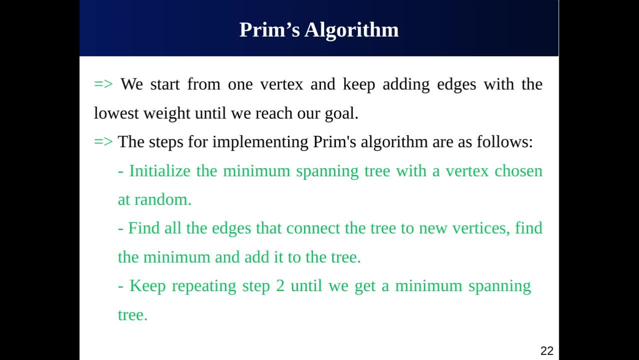 the best solution, what is the optimal solution at that particular instance of time? and then we hope to find a global optimum solution, as we saw in the case of grayscale algorithm. but here we have to start from one vertex, as i just mentioned, not from the edge, but from vertex, and that is the main. 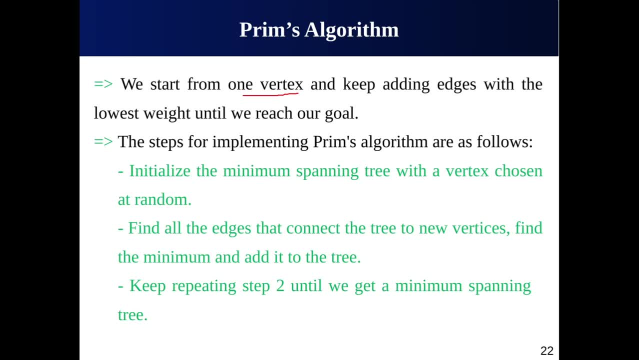 difference between the grayscale and frame algorithm. there we start from the edges, here we start from the vertex or node, and then it is followed by adding the edges with the lowest weight until we reach our goals. so the steps, in summary, are as follow: you have to initialize the 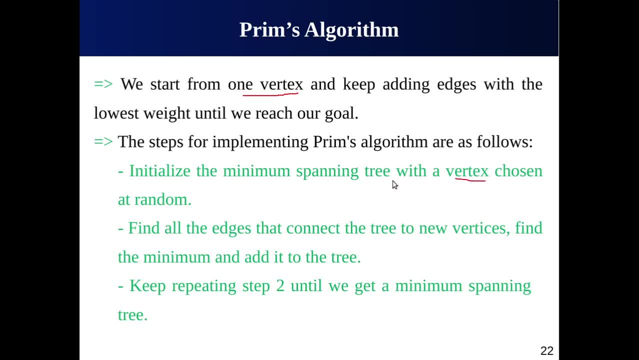 minimum spanning tree with a vertex of your choice, and you can choose it at random. after that you have to find all the edges they are. they connect the tree to new vertices. but the condition is that you have to add a minimum value and then you have to add it to the output or graph and then you have 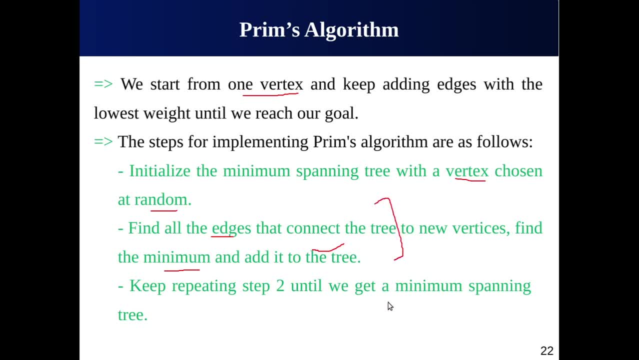 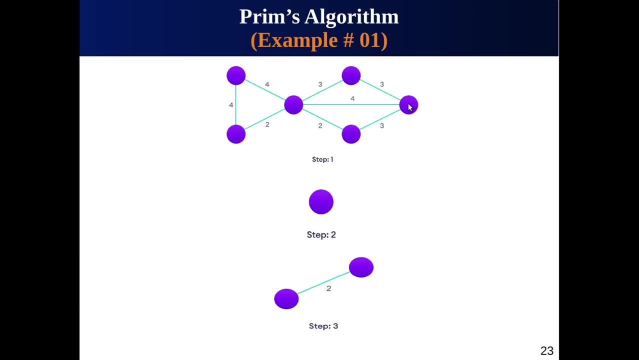 to repeat this step again and again until we get the required minimum tree. let us see an example, similar example, but we are going to apply a different algorithm and there is the frame algorithm. what's going here? the first step is to select, choose, predicts randomly. suppose we have. 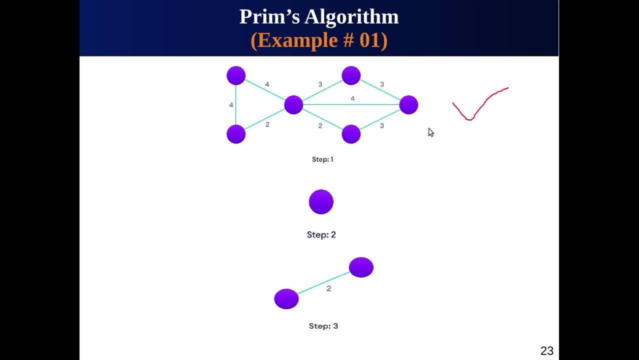 given to us this graph. if a question come in the examination, the graph will be given. the weights should be here, or maybe the weights are given in a table? okay, then you can put the weights edges. the first step is to choose any node randomly selected node. let's suppose the node that we have selected is this one, node a. 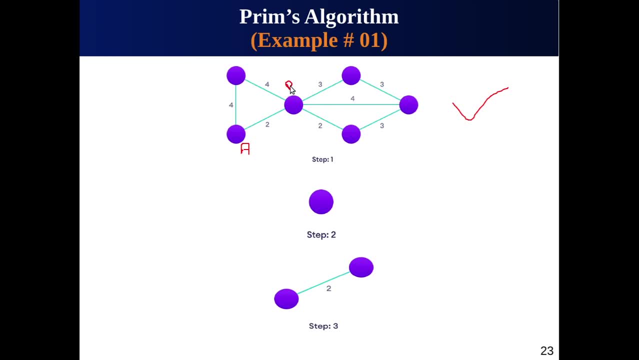 sorry, the nodes have. the cost from a to b is the next thing is simple: choose the nearest vertex from here or here, from a or but the vertex should be the one that is not actually part of the solution or that has not been selected. so if you see the, the edge with 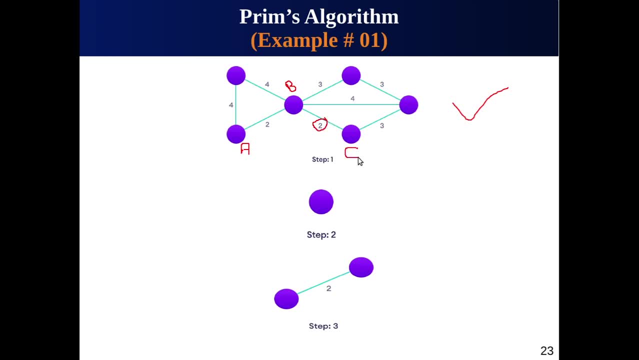 the minimum number is this one? suppose this is, so we have to make it part of, we have to make it part of solution, and then, from date particular, note the nearest edge not yet included in the solution- and if there are multiple choices available, choose one at random. 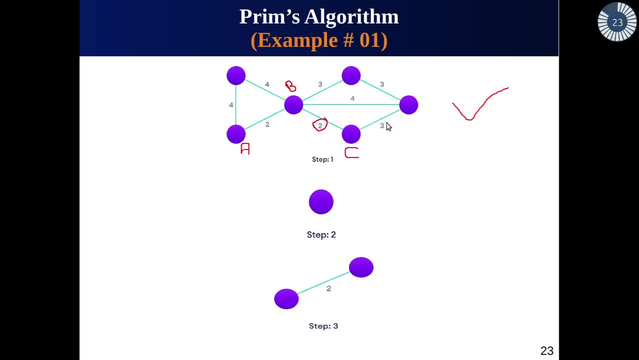 at your own choice. so if you see from here, you have three, we have three. I have selected this one be part of the solution and there is many overhead. next, to give attention, the minimum value is here: three, there is make part here and after date, uh, it has been done directly. the next one is uh with the weight. four, that is here. 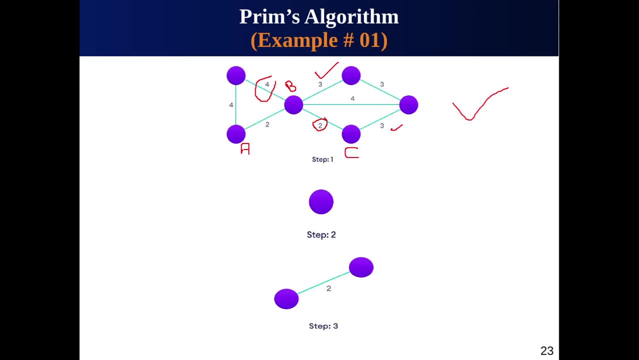 so this is actually a part of solution, and then we will get a spanning tree like this. let us see the second example. the second example is: all always is almost the same, as we saw in the case of crystal algorithm. uh, but here we have to start from any, from any vertex. 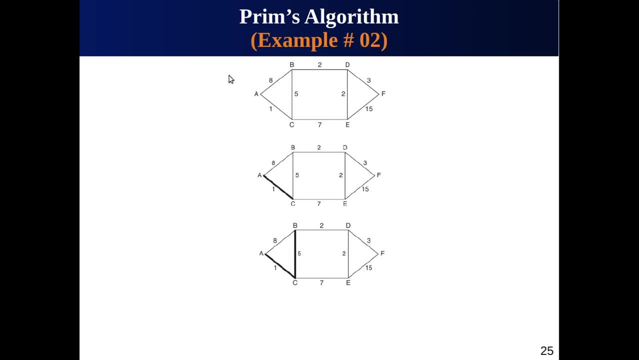 from any node, not the edge. suppose we start from a. this is our starting. we have selected a to be the starting vertex now, since from amongst all the edges that leave the node a, for example a to c and a to b- the smallest edge value or the edge with the smallest value is ac, because the value here 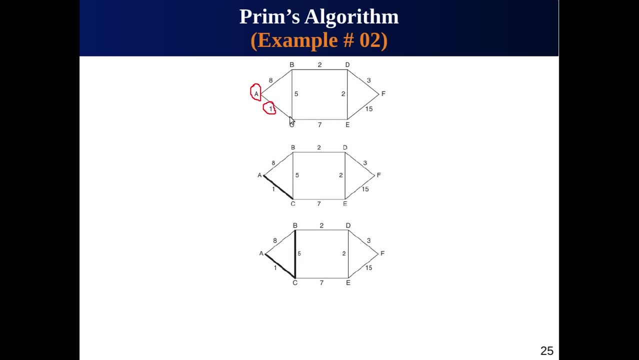 is one that is the least cost. so ac has been selected and you can see it here. the dark line show that we have selected ac and it is now part of the solution in the next iteration of this prime algorithm. now you have to select the edge which has the least cost. the active nodes now are a and c, the edge from a to b. 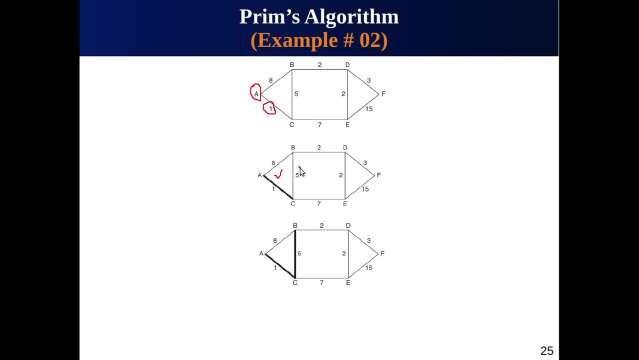 has a cost of eight, the edge from c to b has a cost of five and the edge from c has a cost of seven. what is the smallest value between three, five? so we have selected this one: r, a, b. as you can see, the smallest now is two. you have to select this one now, the smallest here. 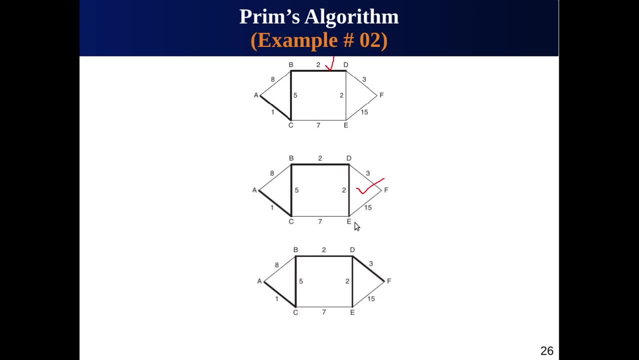 is two, so d- e has been selected. next, the smallest value is from d to f, so this one has been selected. okay, i think we are done. oops, because all the vertices are now connected and we do not have any there. let us see animation of the print. 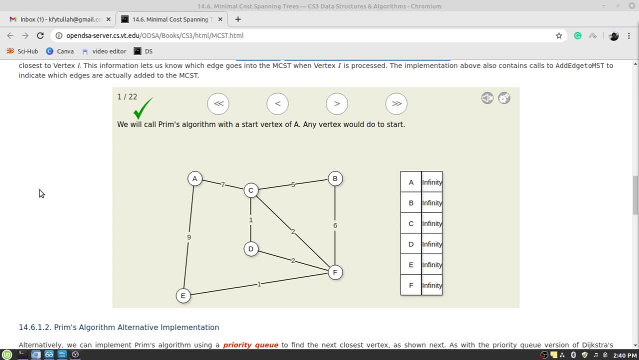 here we have animation. uh, as i just mentioned, prim is simple to code, simple to implement, and here you can see we can implement it in by using a simple array or word, simple array of vertices. let us see we have a graph given. the first step to do is to select any arbitrary node. 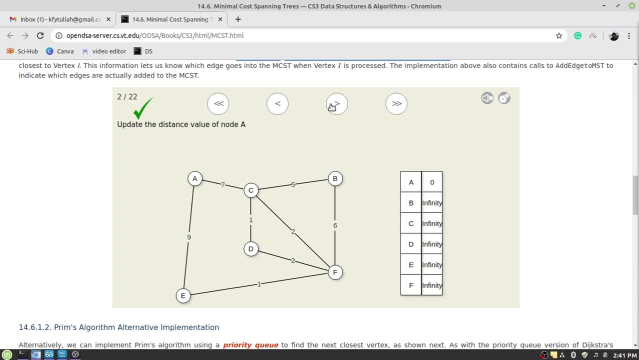 randomly. of course, we have selected a. okay, now you have to select the edge from a, which has the lowest value. so from a to e, the cost is nine, but from a to c, the cost is seven. obviously, we have to select the c. the next vertex is c and the 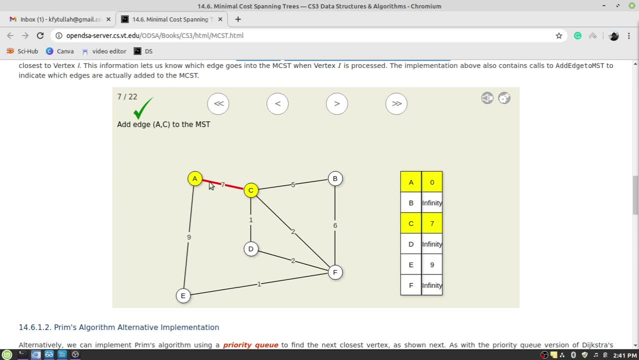 cost is seven. okay, so make it part of the solution. now the active vertices are a and c. the cost is nine. here, here, the cost is one. there is obviously the lowest, the least cost. so make a, c to d the edge part of the solution. so d is selected, now the cost is one. make it part of the solution. give it dark. 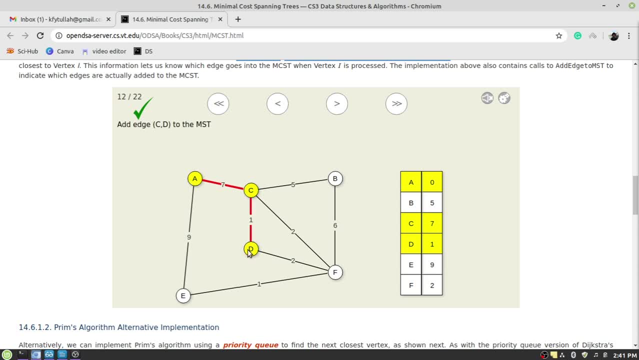 color: red, dark color. that's it. now we have three active, uh, three active nodes. let us see the cost. the cost from a to e is nine, from c to d is. from c to b is five. from c to f to: from d to f to both have equal chances of selection. you can either select: 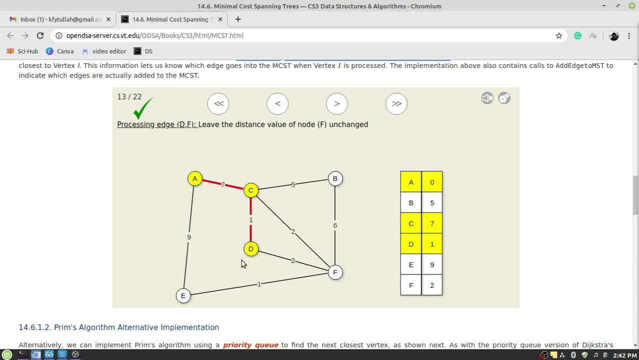 e to f or d to f. let's suppose we have selected d to f, so the cost f is and the link. sorry, they have selected c to f, not doesn't matter. so c to f, the cost is two and that's it. next you have to. 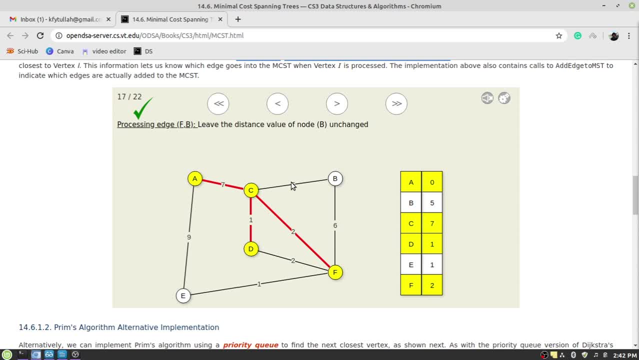 find the, the edge that has not been selected yet and that has the lowest or least cost from a to e. the cost is not c to b, the cost is five. f to the cost is six. f to e, the cost is one, that is the choice, f to e, one selected. next one step. 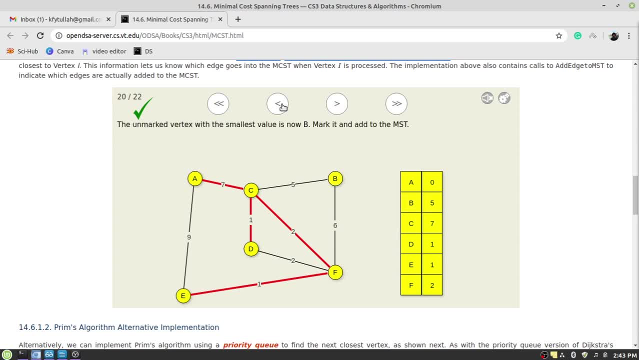 forward. uh, okay, uh, you. now you have different options from a to e. that is not possible. why? because the cost is very high and also it we. if we make it twice, then it will lead to cycle. next we have two options: e to b and f to b. the least cost is from c to b, so there is going to 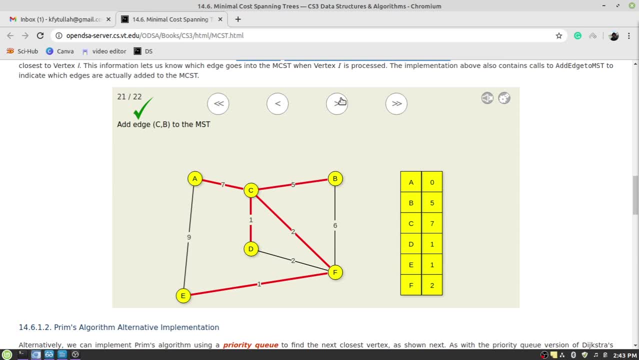 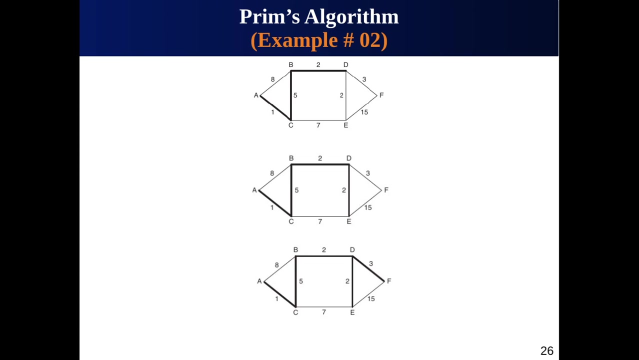 be the choice and that's it. we have covered all the vertices and the. the resultant- uh minimum spanning tree is like this: the other directions, okay guys. uh, this was about greedy approach. uh, optimization problems, fiscal and prime algorithms, things like that. let me conclude the lecture. okay. so in today's lecture, uh, we studied about the greedy approach. 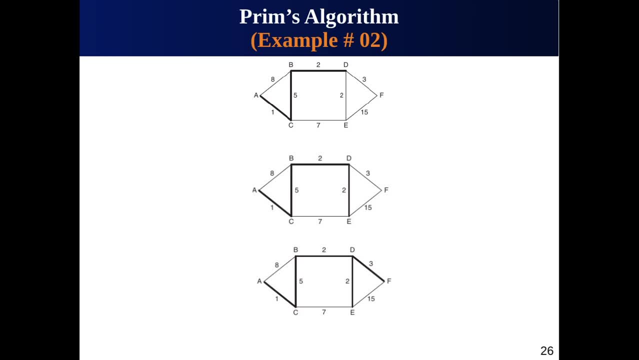 and about the minimum spanning tree, fiscal and frame algorithm in some way. let me conclude like this: if you have given a connected and undirected graph like this, this is actually a connected, undirected graph. a spanning tree of this graph is actually a sub graph or a tree. you can say. 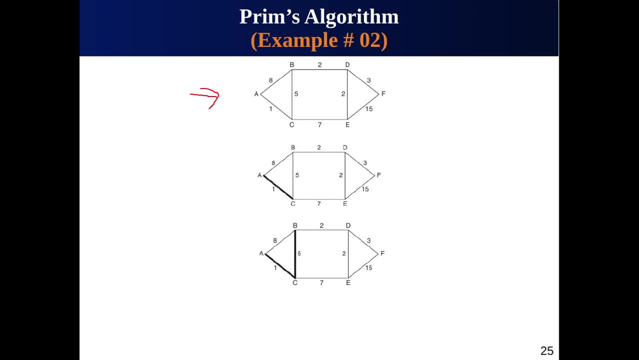 which actually connects all the vertices together, connected graph and there will be no cycle, an edge, starting from the node and ending at the same node. that is like a cycle or you can see circuit the loop. second important point: that a single graph can have many different spanning trees. now we are interested only 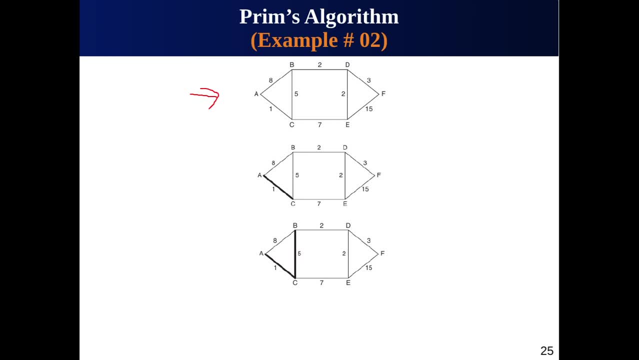 in one solution. so the minimum spanning tree or minimum cost spanning tree or minimum weight spanning tree for this graph is actually a solution that also lead to a graph which is connected, fully connected, and the graph is also undirected, but it will have the least weight. for example, if you have 10 spanning trees for a graph. so what is going to be the minimum? 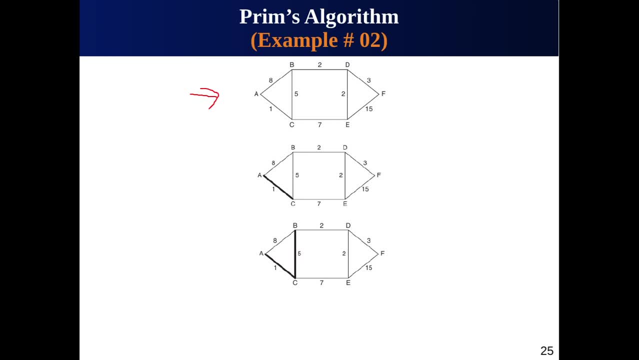 spanning tree, amongst them, the one which lead to the least weight among them. so the weight of a spanning tree, as you know, is actually the sum of the weights given to each edge of spanning tree. you add all the all the cost, all the weights, all the costs, all the costs, and you can see that the weight of the spanning tree is the. 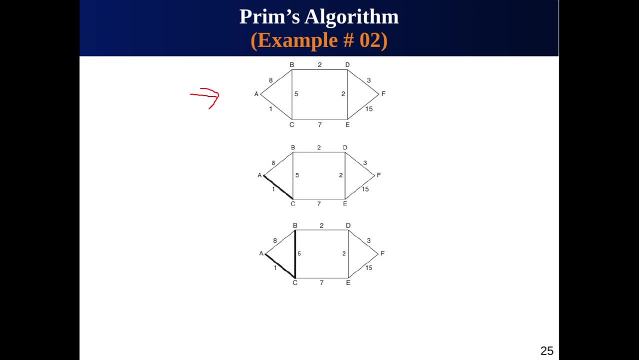 the individual edges and then you get a sum of the weights. date sum must be less from all, from all the from all the sums of the other spanning minimum spanning tree, from the other spanning tree. sorry, used, let me revise: if you have a graph like this, then several. 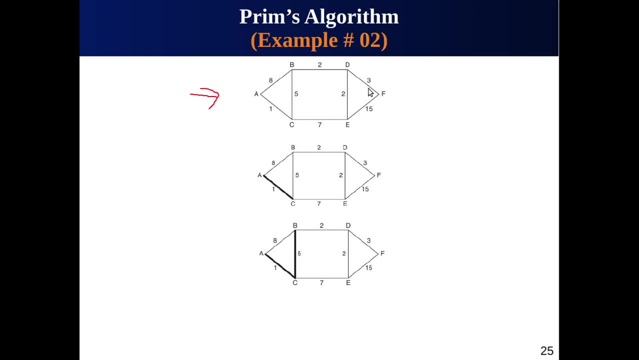 spanning trees are possible, but we are interested only in a particular spanning tree. what is that tree? that tree is known as minimum spanning tree or minimum cost spanning tree, or minimum weight spanning tree. that is actually a tree, a graph that is weighted, unconnected and undirected, without any. 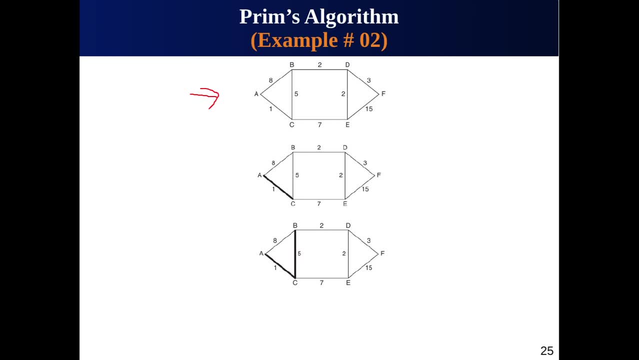 cycle and the total weight of date spanning tree should be less than the weight of all other any. in order to find a minimum spanning tree, we can actually use different, like brim, like griskell, their famous algorithms. date actually uses the greedy approach, or you can say optimization- they work towards optimization, both the prime 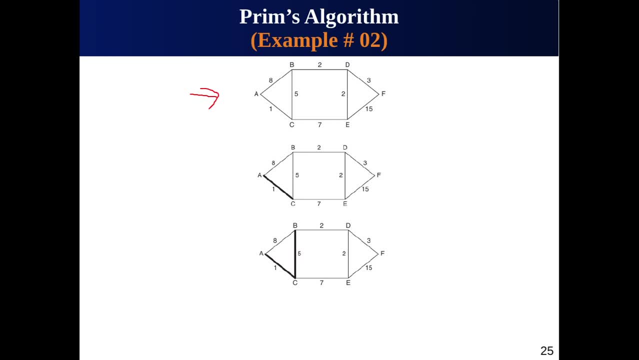 and crystal algorithm are greedy algorithm and they are used for finding the minimum tree. Remember, both the PRIM and Kruskal algorithm are actually greedy algorithms and they are used for finding the minimum spanning tree, But you can apply these algorithm on graphs that are weighted, that are 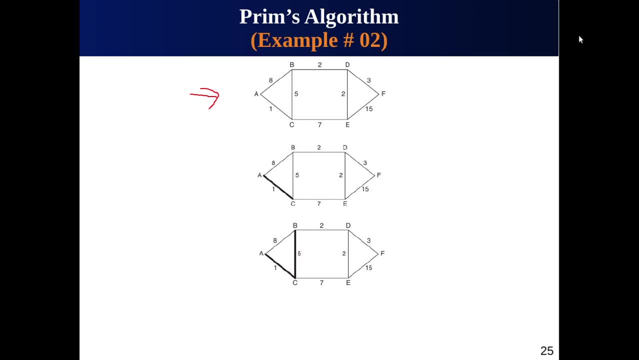 connected and that are undirected. Finally, there is a difference between the Kruskal and PRIM algorithm. The main idea behind the Kruskal algorithm is to sort the edges based on their weights. Remember, we focus on the edges- and then, from implementation point of view, first we 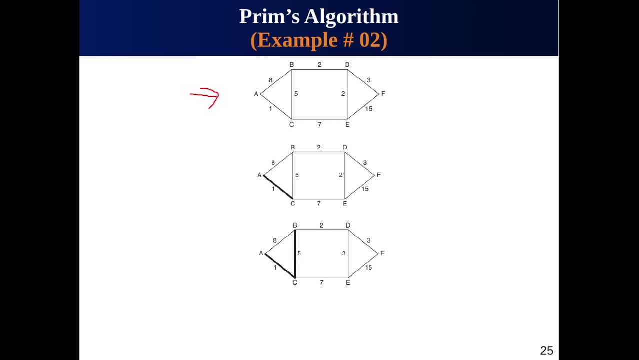 need to sort the edges in ascending order from low to high. After that, we start taking edges, one by one, based on the lower or least weight. In case we take an edge and it result in forming a cycle, then what we need to do This edge? 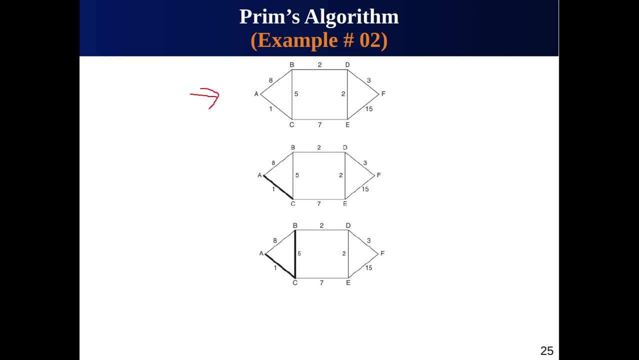 is not included in the resultant MST, Ignore it. But if it does not lead to a cycle, then we include it in the resultant MST. On the other hand, the PRIM algorithm is actually a modified version of the Dijkstra algorithm or test pathfinding algorithm. Here in PRIM algorithm, we 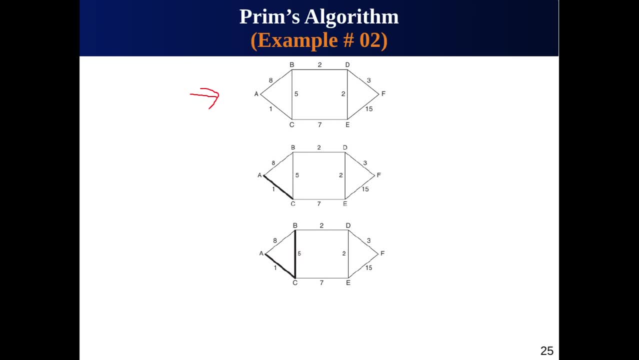 first choose a node, not an edge. We randomly choose a node to start the algorithm and then from there we add all its neighbor to the output solution. We perform multiple steps and in each step we extract the node that we are able to reach using the edge with the lowest or least weight, & therefore you can say that we extract the node, we add them to the next one. 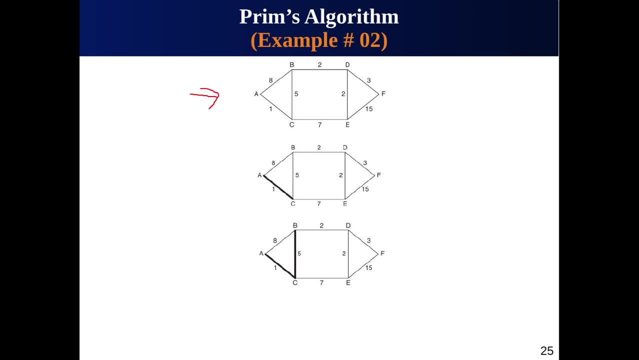 add them to the resultant minimum spanning tree if it does not leave the cycle as it's in case with algorithm. so, in conclusion, the main difference between these two algorithm is that in the critical algorithm we start edge, while in the time algorithm we select any node or any vertex randomly, then we 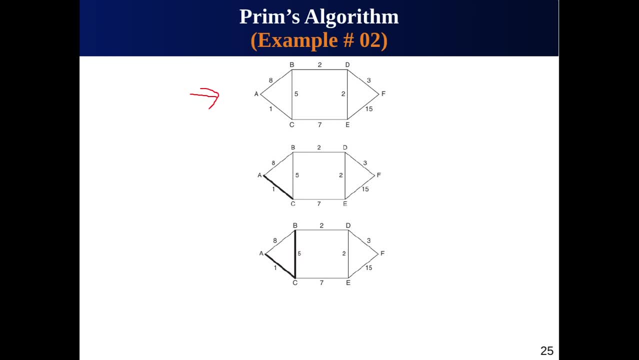 decide. other differences are also there. for example, if all the edges weights are- this is a bit technical, but let me share with you that if all the edges have the same weight- not same but distinct weight- the weights of all the edges are unique. there is no duplication in the weight- then both the algorithms 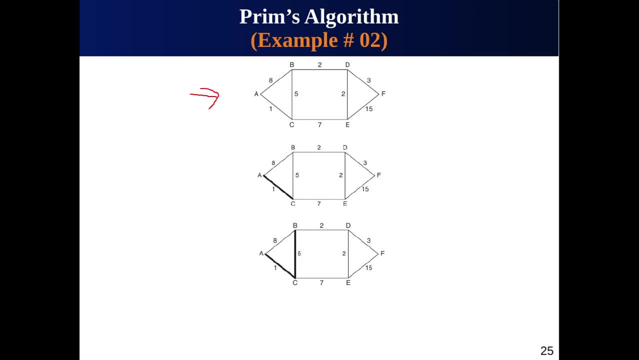 guaranteed to find the same minimum spanning tree, they will lead to the same solution. you can say: if the weights are distinct for the each edge, but if the edges are weight associated with the edges, if they are not unique, they are not distinct. then both the algorithm may not always produce the same MST. however, in both the cases 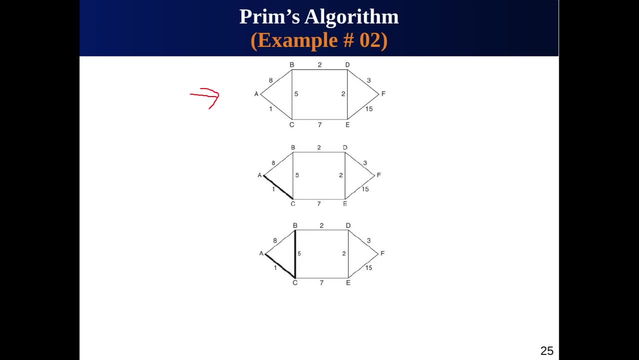 both the MSTs produces by these two algorithms would but would always be the same. so you can see in the diagram. then all the edges are nearly the same, but with the adults there is no simplesmente duplication. on every of these edges there are duplication, there are duplications and 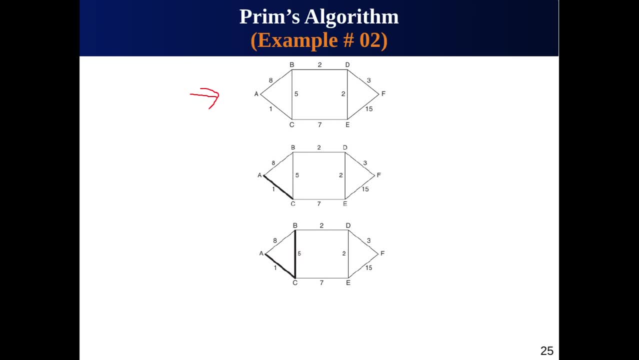 the algorithm may not always produce the same mst. another thing about prime prim algorithm is that it actually initialize with a note, while critical algorithm initiate itself with an edge, as we just okay. uh, from implementation point of view, or from the usage point of view, prim algorithm is preferred when the graph is dense. 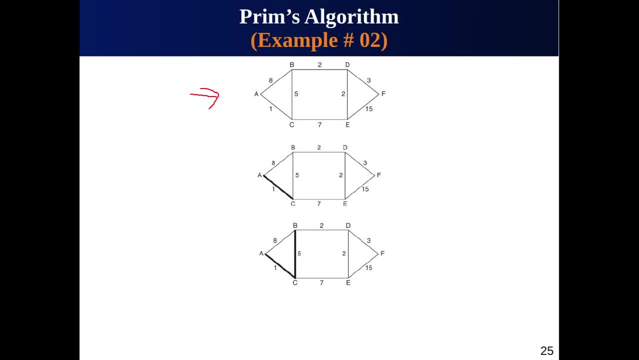 on the other hand, the critical algorithm is preferred when the graph is like a spares with no many edges or or nodes. and finally, there are some other solutions. there are also some other differences between the two algorithms. maybe, if you are interested, you can find on the google about these algorithms.